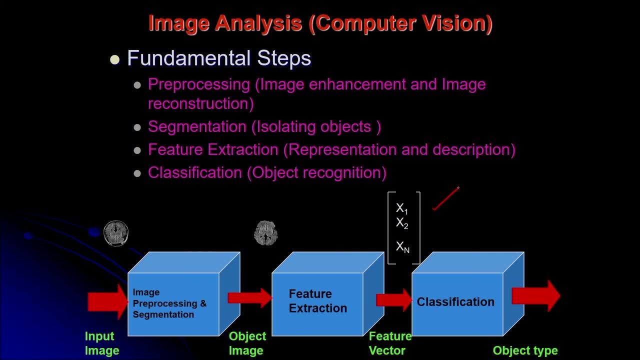 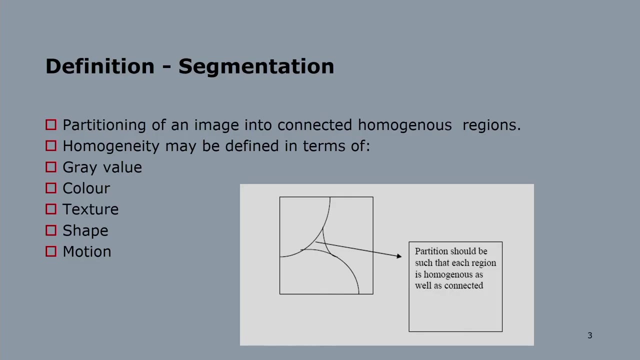 images And this is the feature vector you can see, And after this we can do the classification of the images, Or maybe we can do, we can go for object recognition. So this is a typical block diagram of a computer vision system, the image analysis system. So what is image? 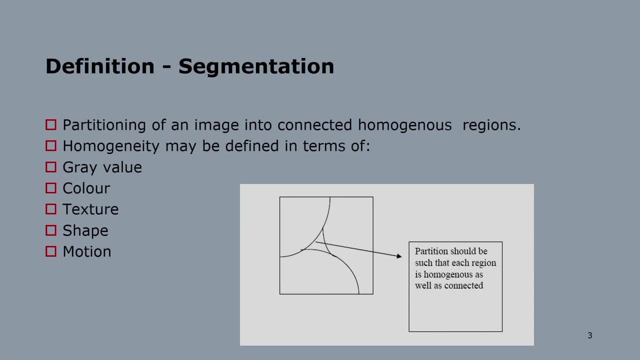 segmentation, Partitioning of an image into connected, homogeneous region. The homogeneity may be defined into in terms of gray value, color, texture, shape and the motion. Suppose if I consider the color, So suppose in this portion the color is almost same, That means it is homogeneous. 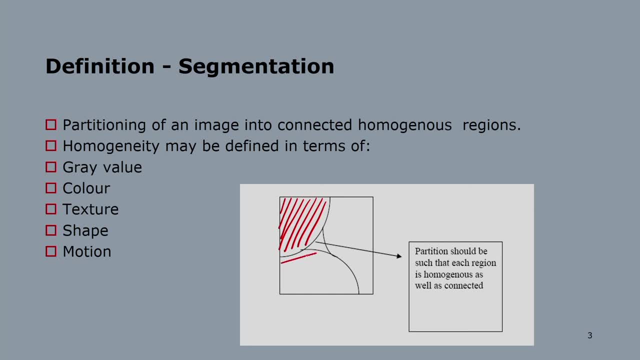 Similarly, if I consider that this region, corresponding to this region, the color is also almost same, That means it is homogeneous. So that means, based on this, the gray value, color, texture, shape and the motion information, I can do image segmentation Here. I have shown one example of image segmentation: My input. 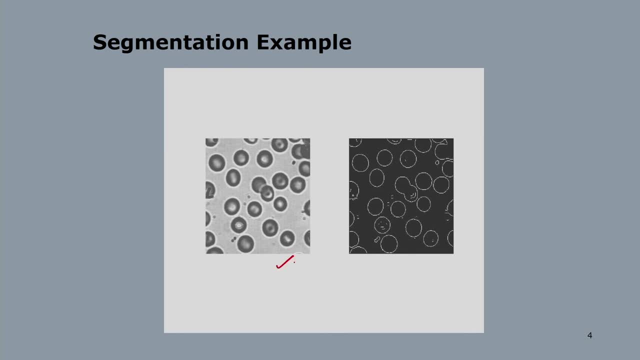 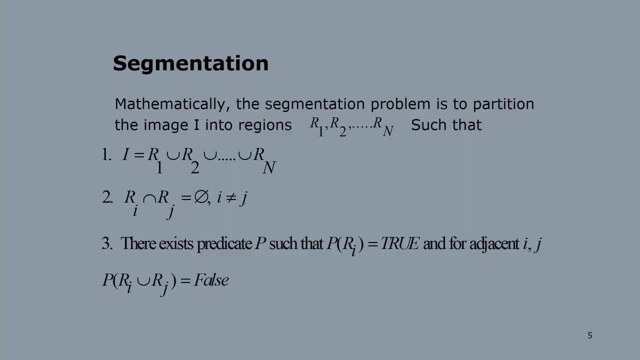 image you can see. the first is the input image, The second one is the segmented image, the segmented output. So, for segmentation, how to define mathematically, The mathematical definition of image segmentation? So, mathematically, the segmentation problem is to partition the 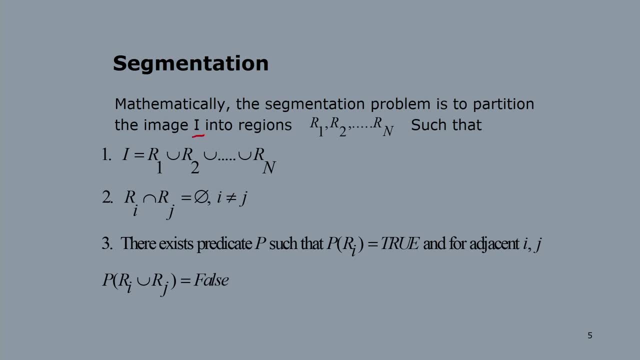 image i. So I am considering the image i into regions. The regions are r1, r2, r3, r4, r5, r6. into regions. The regions are r1, r2, rn, like this. So i is equal to r1 union, r2 union. 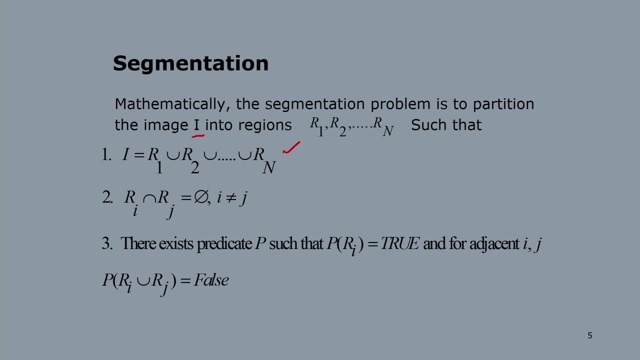 r3 like this. So that will be my image. And in this case, if I consider ri- intersection of rj- two different regions- then in this case it will be phi. the null set i is not equal to j, So this region is defined like this. That is if I consider all the regions. 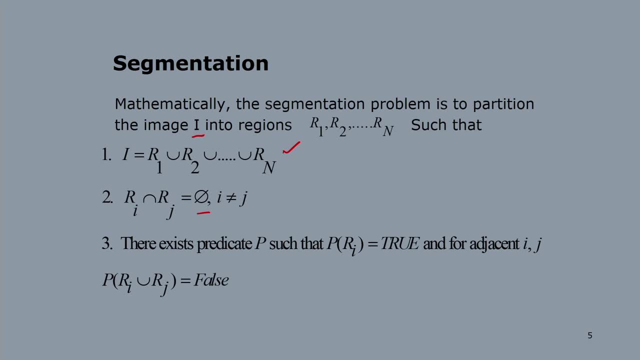 then I will be getting the image. And if I consider two different regions, that means in this case ri intersection with rj will be phi, For determining the homogeneity. I am considering one measure. That measure is called a predicate, So predicate of a region, the predicate of a region, is true that I have. 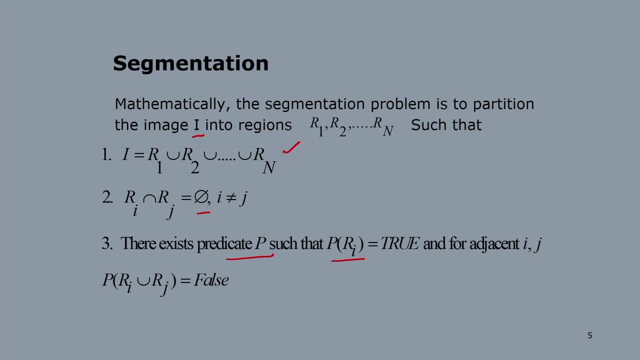 considered for the homogeneous region And in this case, if I consider the adjacent regions, that is, two regions, ri and rj, the predicate of ri union rj will be false, that because it is not homogeneous. So based on the homogeneity I am defining this term, the term is the predicate, So for 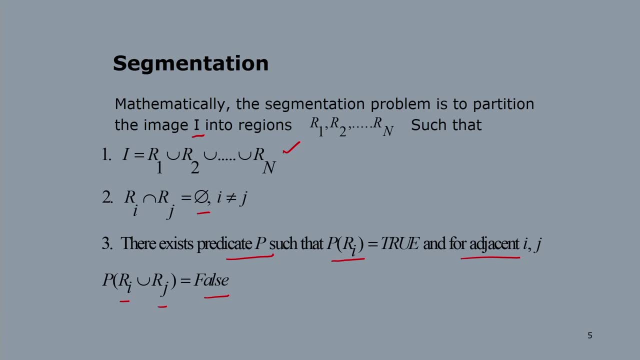 the homogeneous region, the predicate will be true and for the nonhomogeneous region the predicate is false. So this is the mathematical definition of image segmentation And, based on the predicate, whether a particular region is homogeneous or not, the homogeneous. So in this class I will discuss these techniques. 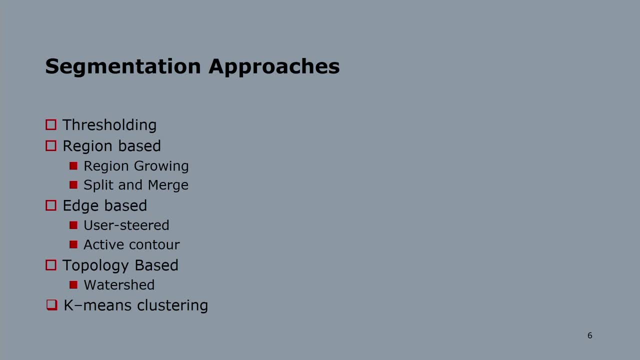 One is the thresholding technique, One is the region based technique, that is, region growing technique. Another one is the split and merge technique And for the edge based technique, I will discuss the active contour based technique And for topology based approach, I can discuss the watershed algorithm. 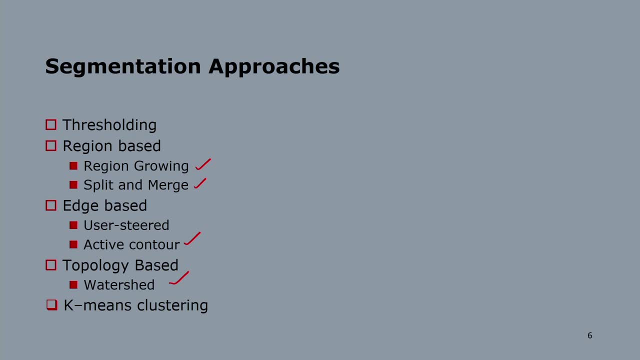 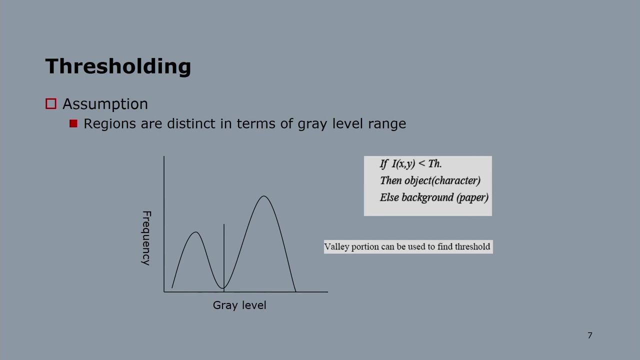 And finally I will discuss the k-means clustering algorithm for image segmentation, For advanced segmentation, principles that I will discuss when I will discuss the computer vision applications. So first one is the thresholding. So here you can see the image histogram I have shown. 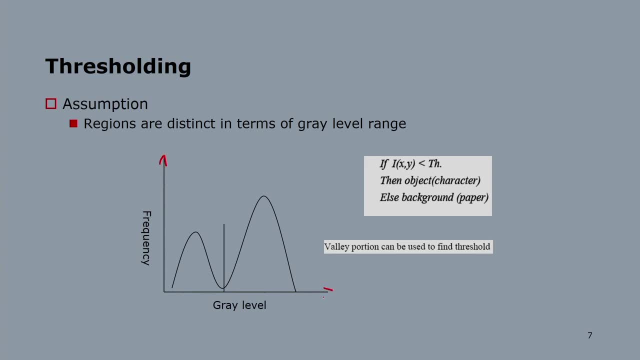 So this side is the frequency and this side is the gray levels, all the gray levels, And based on this algorithm you can see: if Ixy is less than threshold, Then object is character and else the background is paper. So in this case, what I am considering- suppose one paper is there, okay? 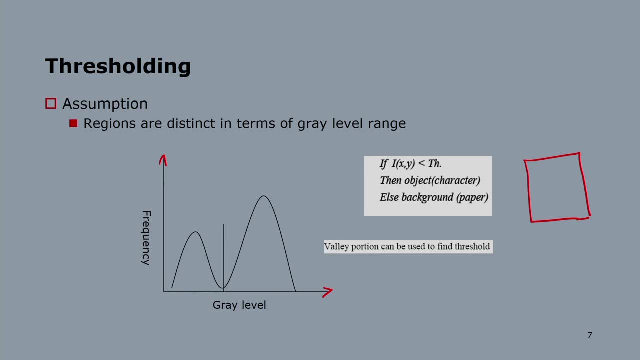 So the background is white background, suppose, and I have the characters here. I am writing some characters in the papers. that is the black. So in the histogram you can see this portion is the black portion And you can see the white is this side. 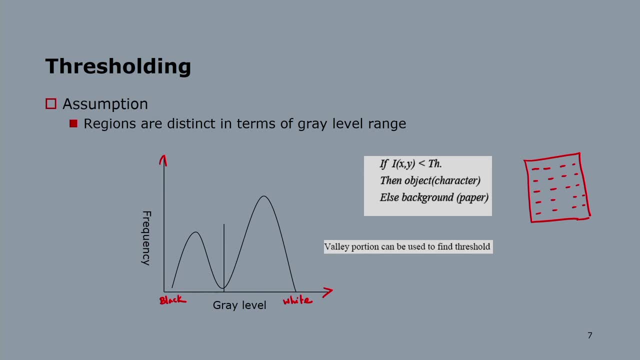 So in this case you can see number of pixels in the black that will be less than the black, the number of pixels of the white region, because white is the, basically the background. the background is white And if I consider the characters, that is the black. 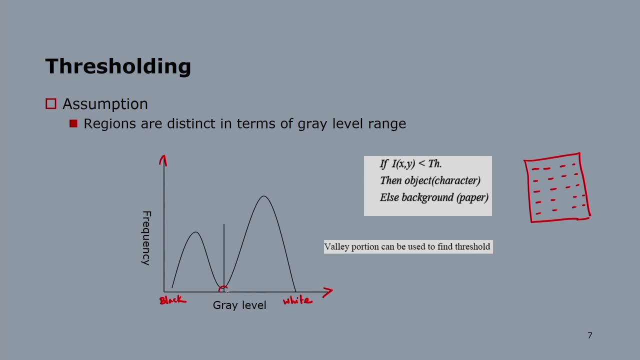 So, based on this algorithm, if you select the threshold, at this point the valley portion can be used to find a threshold. So suppose, based on this, if I select the threshold, then what I can do, I can separate the objects, that is, the character, from the paper. the paper is the background and corresponding 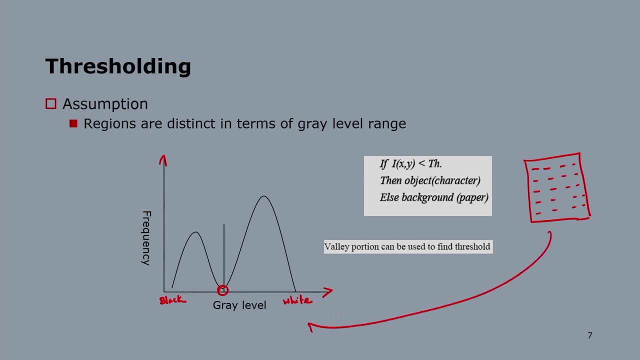 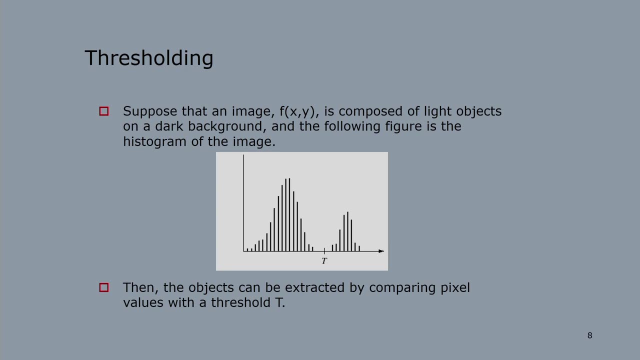 to this case And this is my histogram corresponding to this case. suppose that an image FXY is composed of light objects on the dark background. So here you can see this is the dark and this is the light. So I am showing the histogram. 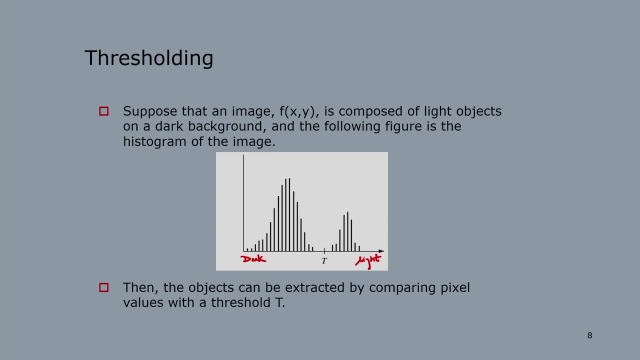 So the image is composed of light objects on a dark background and corresponding to this, this is the histogram. Then, if I consider the threshold at the valley- T is the threshold- suppose then the objects can be extracted by comparing a pixel values with a threshold. the threshold is T. 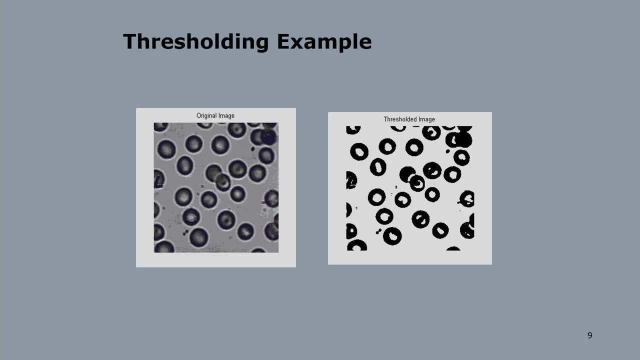 So this is the principle of thresholding and, corresponding to this principle, you can see this is the input image, original image, and after this I am applying the thresholding principle and you can see the thresholded image you can get as an output image. 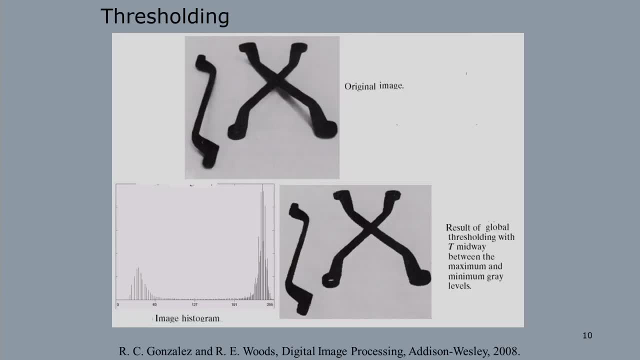 Again, in this case, this is another example of the thresholding. You can see the original image and, corresponding to this original image, you can see the image. 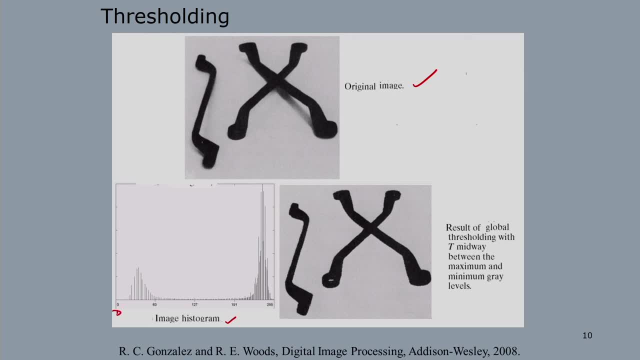 histogram, and already I have mentioned this is the dark side And this is the light side. this is the light side, that is the background and object is the foreground. that is the dark. So you can see the number of pixels in the light portion is greater. 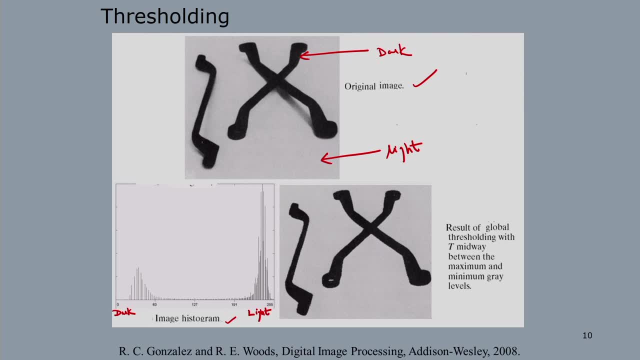 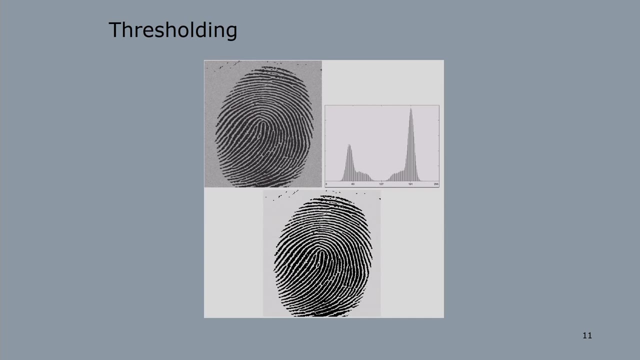 than number of pixels in the dark regions. and if I apply the the thresholding principle, then, corresponding to this, you can get the segmented output like this: so this is the segmented output and this is another example of thresholding, that is, the fingerprint segmentation. so, corresponding to this input image, this is my histogram and I can select the threshold. 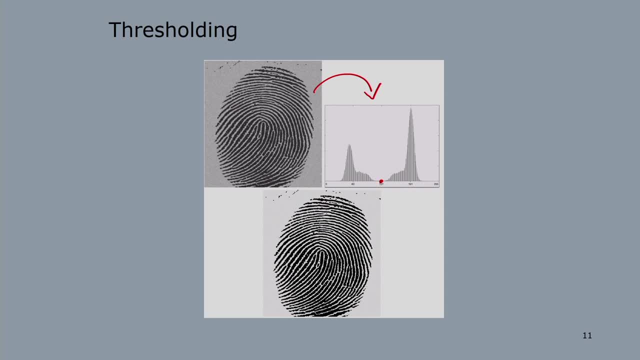 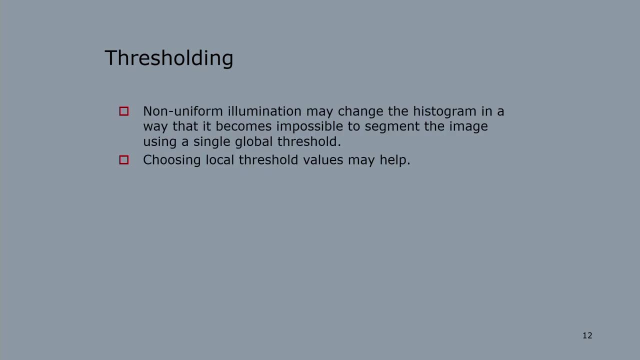 suppose here and based on the threshold, I can do the segmentation, the segmentation of the fingerprint from the background. that I can do. but the problem of the thresholding is that non-uniform illumination may sense the histogram. that is the one problem. so that is why it is very 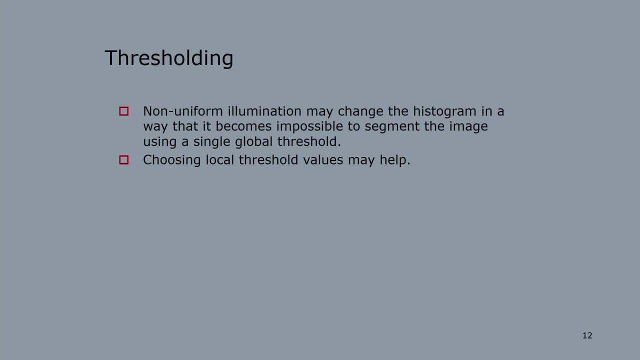 difficult to segment the image using only one global threshold. so for this we have to select the local threshold. maybe we have to select, so that is the problem with the thresholding. then, in this case for the non-uniform, illumination can sense the histogram of the image and in this 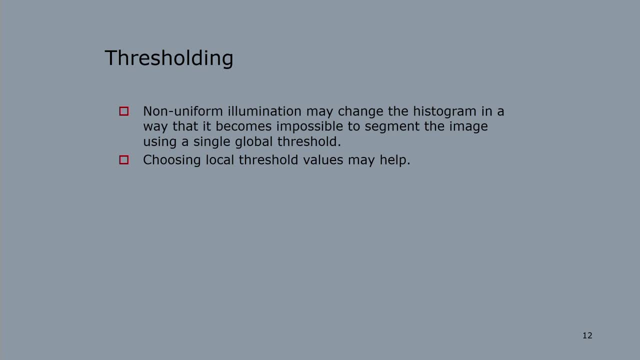 case it is, you can see that the image is segmented. so that is the problem with the thresholding. it is impossible to segment the image with the help of single threshold, so that is why we have to select local thresholds that we have to consider. so in this case, you can see. 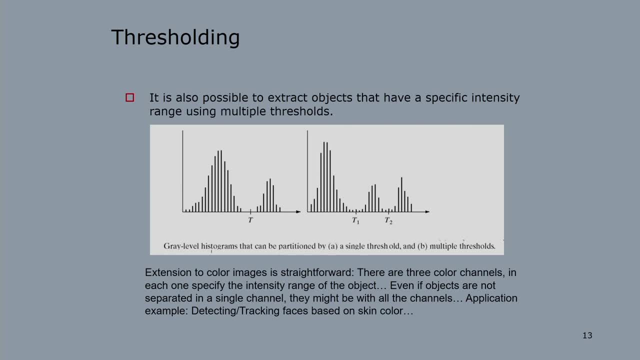 the gray level histograms I have shown, and you can see in the first figure I have shown only one threshold. in the second figure I have shown two thresholds, t1 and t2 for segmentation. so this principle can be extended for color image also, because the color image has three channels. but already I have defined the r, g and b, three color channels. 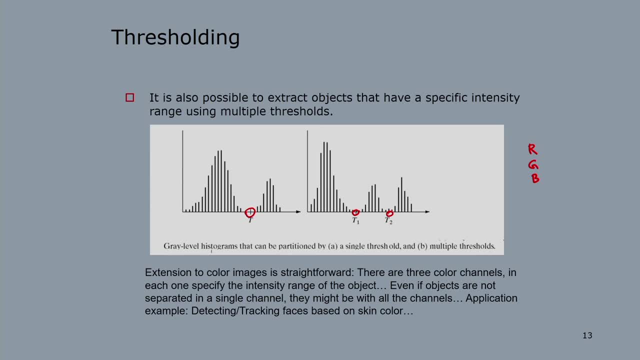 so suppose, even suppose one object which is not separated in a single channel. suppose it is not separated in the single channel. suppose in the r channel it is not separated and that might be separable in other channels, suppose corresponding to g channel. if I consider the g channel, the separation is possible, the segmentation is possible. 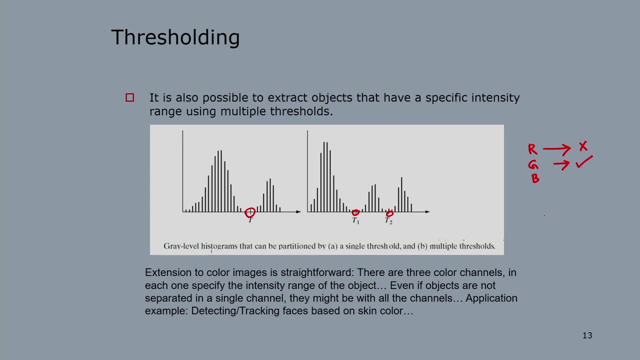 In case of the r channel, the objects cannot be separated in a single channel, so that is why we have to consider all the channels. so this is one application that is detecting, tracking faces based on color, the skin color. so for this I have to consider r, g, b channels. 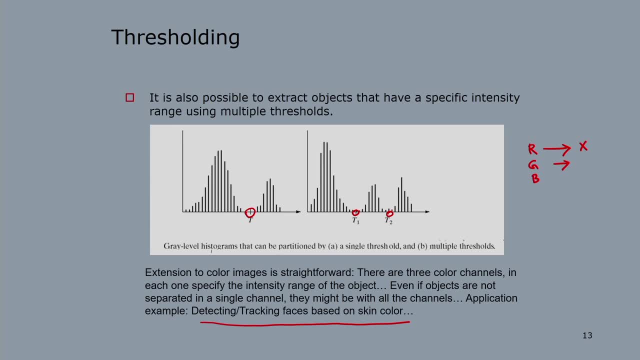 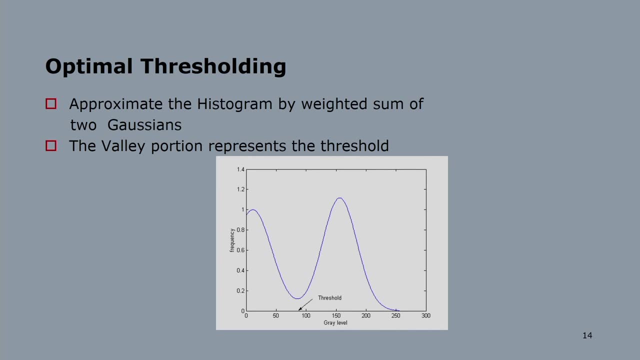 the red channel, green channel and the blue channels for the color image. another technique is the optimal thresholding. so in this case, approximate the histogram by weighted sum of two gaussians. What I can do. the valley portion represents the threshold, so threshold can be selected from the valley portion and this is called the optimal thresholding. 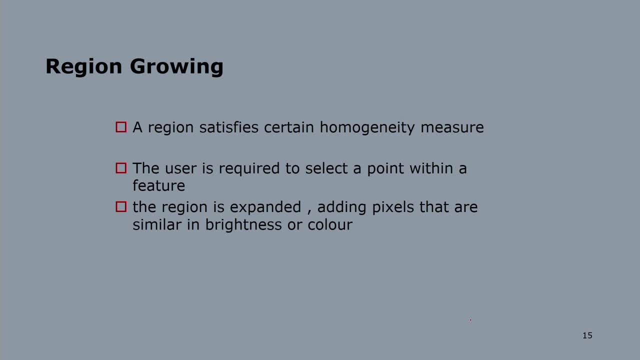 Now I will discuss another technique, a region based technique, that is, the region growing technique. so for this, what I have to consider a region satisfies certain homogeneity measure. so already I have defined the homogeneity in terms of gray value, maybe in terms of color value, maybe in terms of texture value, like this. so this is based on these parameters. 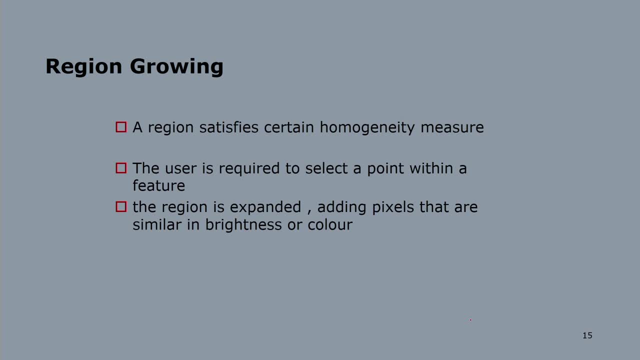 these attributes, that is based on the color information, based on the gray value, based on the texture information, I can define the homogeneity and in this case the user is required to select a point within a particular feature. that means suppose within a particular region or within a particular feature, means suppose corresponding to this color, a particular color. 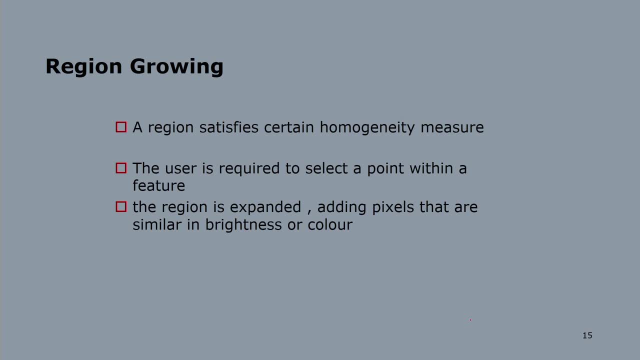 in a particular region. I have to select a particular point. the region is expanded, adding pixels that are similar in brightness. So the concept is like this: suppose let us consider one image, this is the image- and suppose, corresponding to suppose this portion of the image, we have some regions corresponding to. 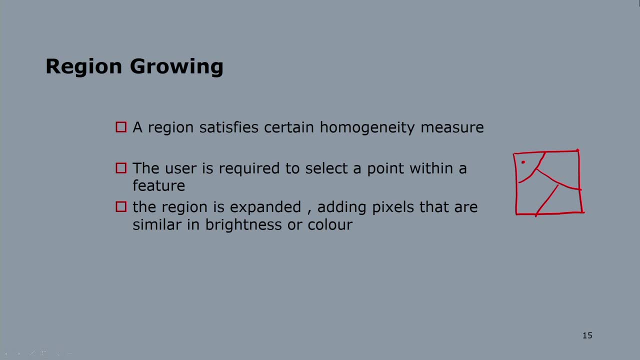 this portion of the image. I am fixing a point, I am selecting a point. after this, what I am considering, I have to compare, suppose, the nearby pixel with this pixel and if the difference in the gray value, or maybe the difference in the color value, is less than a particular 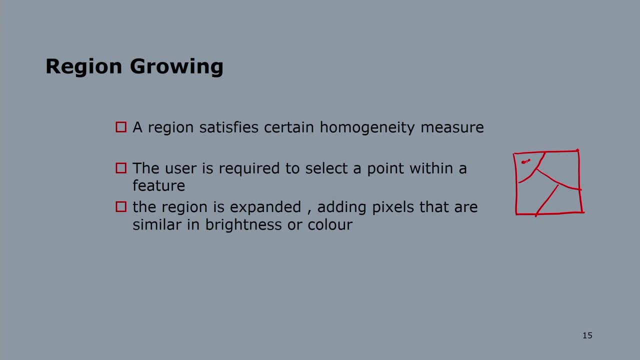 threshold, then in this case- the second point- I can merge with the first point and I can grow the region and, like this, if I consider another neighborhood, I can compare that pixel value with the other pixel value. if this value is less than a particular threshold, then I 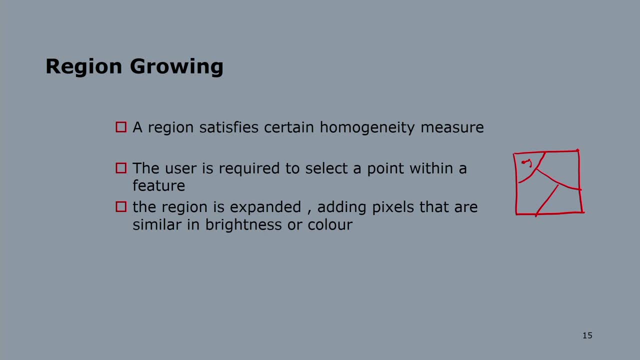 have to merge that one, otherwise I have to neglect that one. so like this, based on this point, I can grow the region in a particular image. I can consider number of such points. so these points are called the seed points. so, based on these seed points, I have to compare the seed point with the neighborhood pixels. if 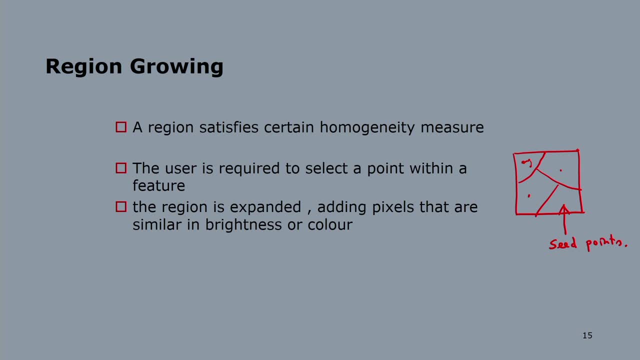 it is within a particular threshold, then in this case I have to consider that point, the neighborhood point, and that is mainly I am determining the homogeneity if the difference in the gray value or the color value of the seed point with the neighborhood pixel is less than a particular threshold. 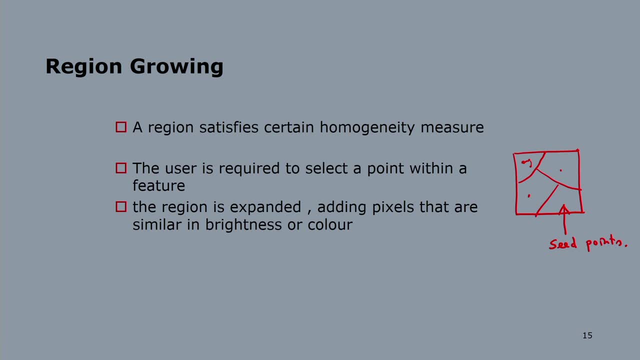 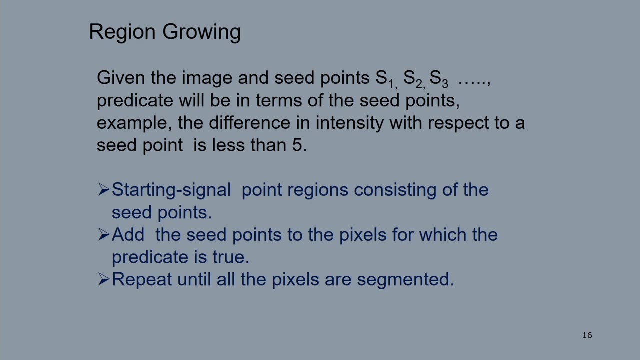 Then in this case I have to consider that point and I have to grow the region. so this you can see in the next slide what I have to consider. so for this image I have to select some seed points- s1, s2, s3- and the predicate will be in term of seed points. 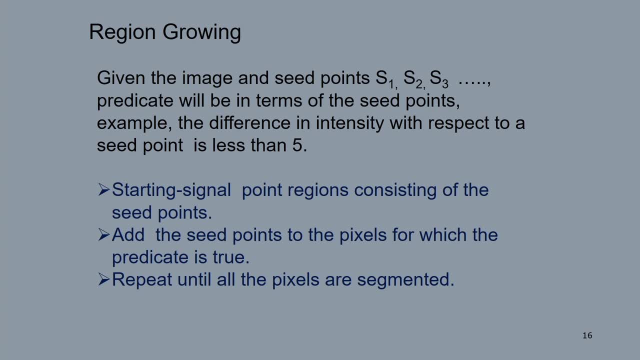 So what will be the predicate? the difference in intensity which respect to the seed point is less than 5, suppose this is one example I am considering. so first what we have to consider: Starting signal point Region Come Below, consisting of the seed points. So first I have to consider the regions with the seed points. 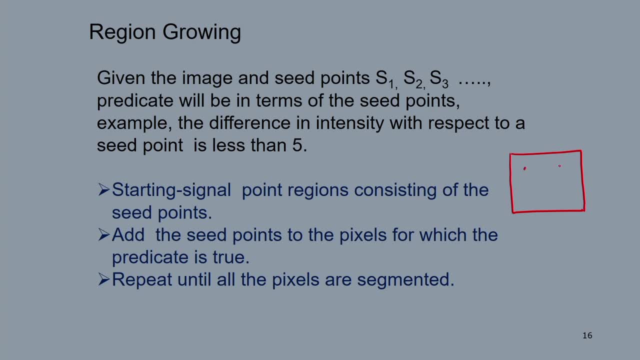 So already I have explained this one. So I have to select some seed points like this: Add the seed points to the pixel for which the predicate is true. So suppose, if I consider corresponding to this seed point, the seed point is S1,. I want to compare the seed point with the. 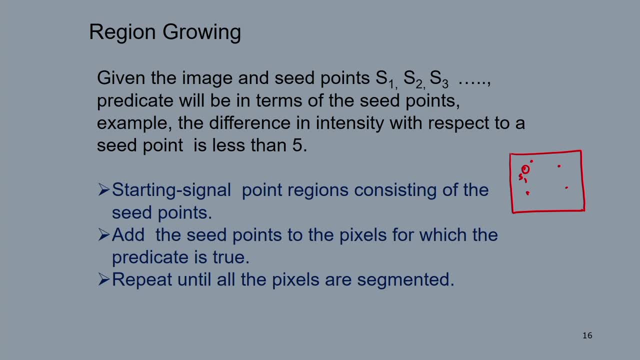 neighborhood pixel. and if the predicate is true, then in this case I have to add the seed points to the pixels like this, repeat until all the pixels are segmented. So I have to do like this In case of the color image. these comparisons I have to make in terms of RGB value. So 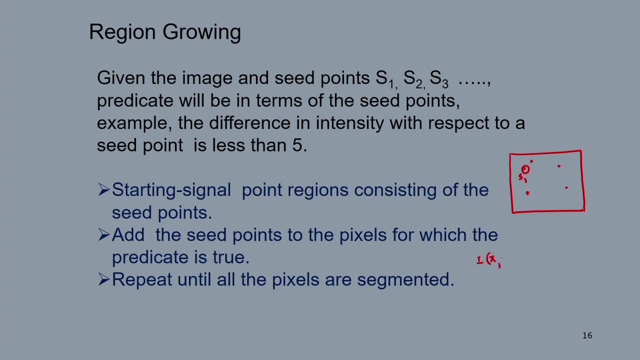 how to compare. Suppose one pixel is suppose the seed point is suppose I XY and corresponding to I XY, the R value is R1, Z1 and B1. That is corresponding to the seed point and I have to compare the seed point with the neighborhood pixel. The neighborhood pixel. 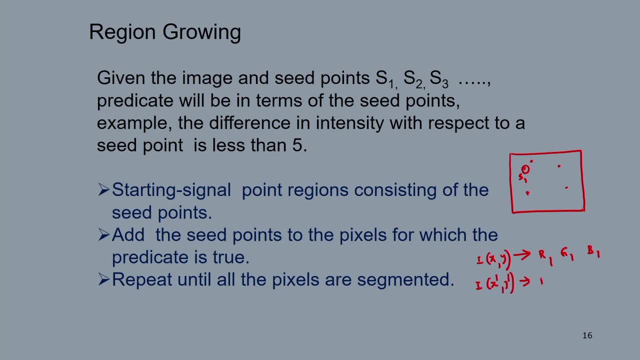 is R1 and B1.. So I have to compare the seed point with the neighborhood pixel. Suppose I, X dash, Y dash, and suppose this value is R1 dash, Z1 dash, B1 dash, and how to compare? So for comparison I can apply the Euclidean distance, So R1 minus R1 dash, whole square. 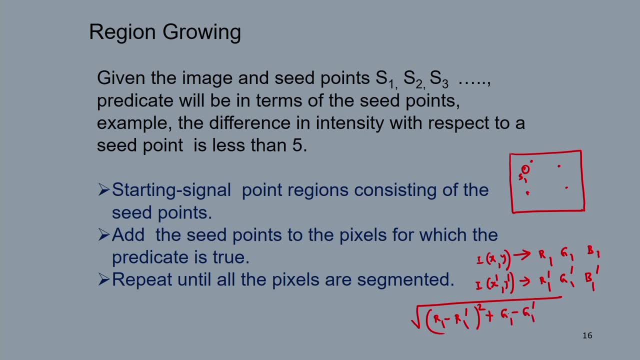 plus Z1 minus Z1- dash whole square. plus B1 minus B1- dash whole square. So like this I can find the similarity between two pixels. That is the predicate I am considering And this predicate is considered to determine the homogeneity condition. Add the seed points. 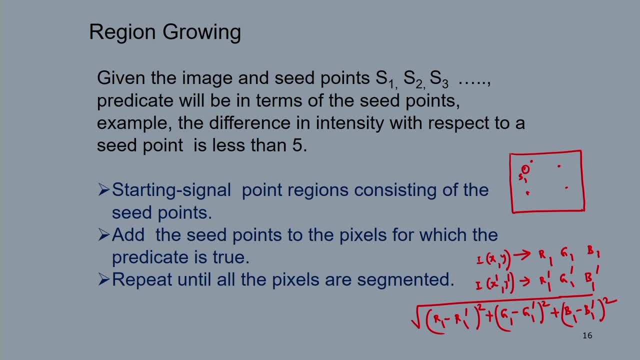 to the pixels for which the predicate is true, And this procedure I have to repeat until all the pixels are segmented out. This is the concept of the region growing. So what are the advantages and disadvantages of this technique? It is a very simple technique. 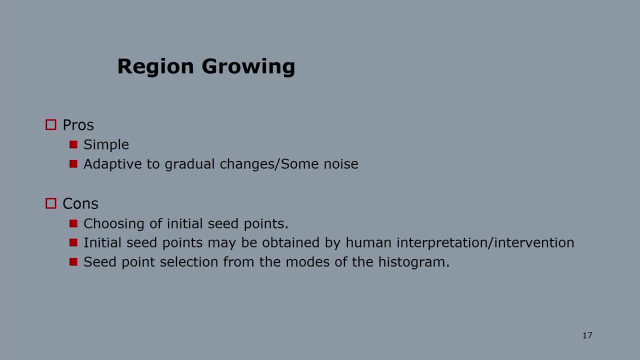 adapted to gradual changes and also it is adaptive to noises. some noises, But the main problem is how to select the seed points, the initial seed points. That is the main difficulty. So initial seed points may be obtained by human interpretation, intervention. Seed point selection from the modes of the 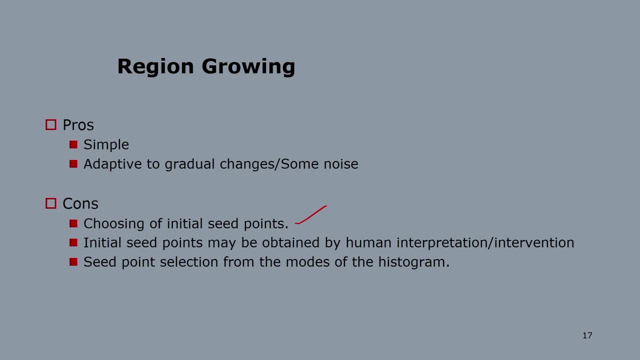 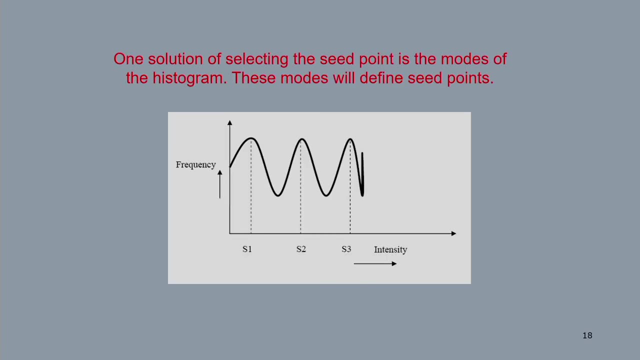 histogram, that can be also done. So I have the histogram and from the modes of the histogram I can select the seed points. So in this case you can see this is the histogram of the image. So what I am considering, I am selecting the seed point S1, S2, S3.. So, selecting the seed point S1,. 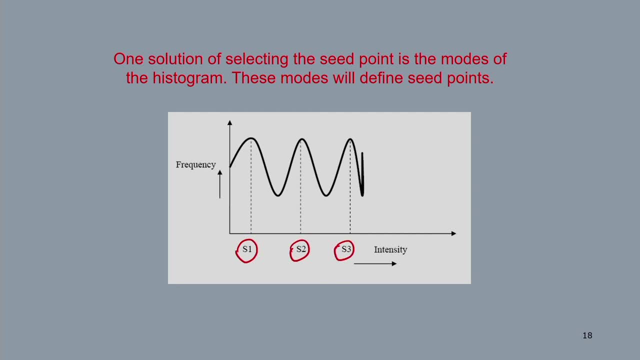 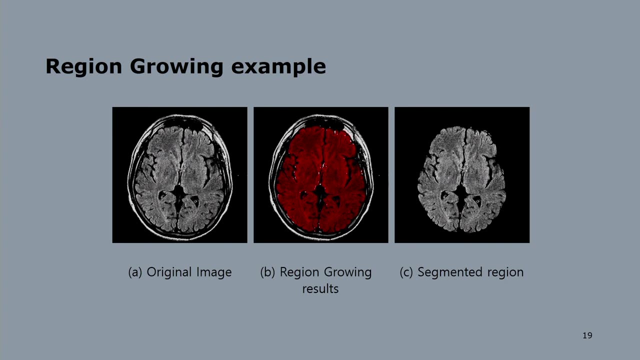 S2, S3 from the modes of the histogram. That is one technique And this is the one example of region growing segmentation technique. So I have shown the original image and you can see the region growing results. For this I have to select the seed points, Maybe. 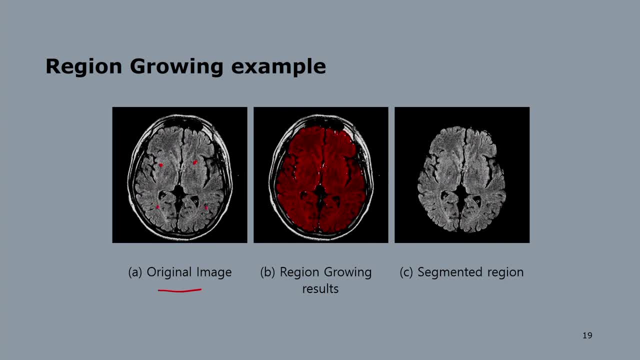 some points like this. we can select some seed points. After this I have to grow the regions. I have to do an iteration 5, that is an iteration 20,, 40,, iteration 30, and this is my final segmentation and finally I am getting the segmented region like this in the final image. So in this case, 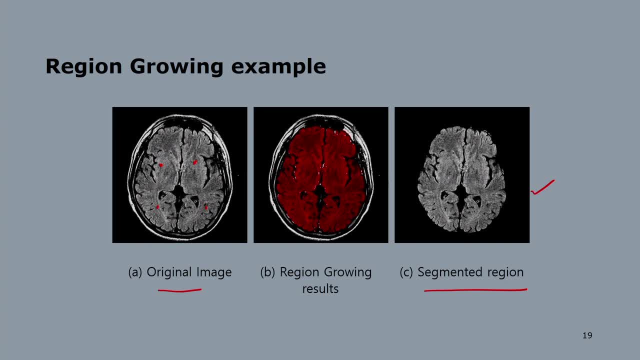 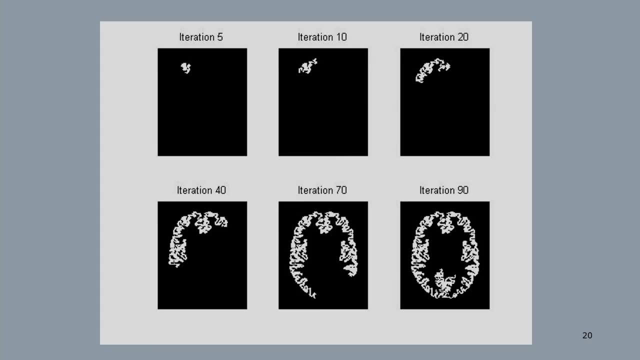 manually. I have to select the seed points in the image, or maybe I can consider that technique, That is, the, from the modes of the histogram I can select the seed point. After this I have to grow the region to do that segmentation In this case. I have shown one example. I have shown iteration 5,. 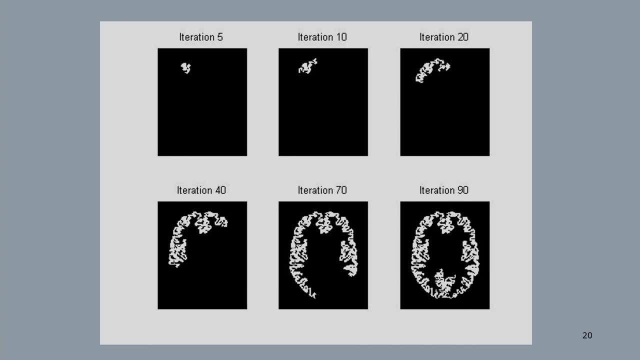 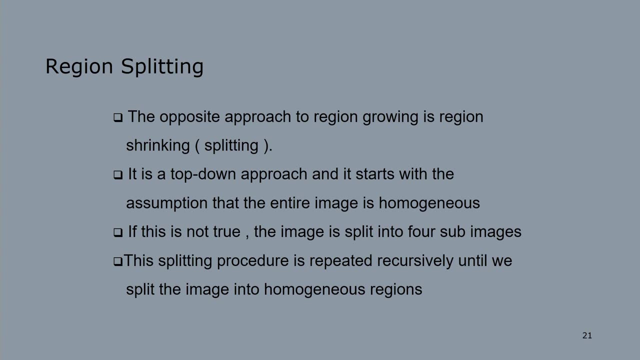 iteration 10, like this: 20,, 40, growing the region and finally I am getting the segmented output after iteration 90. That is one example of that region growing technique. The another technique that is also another very important technique, that is region splitting. 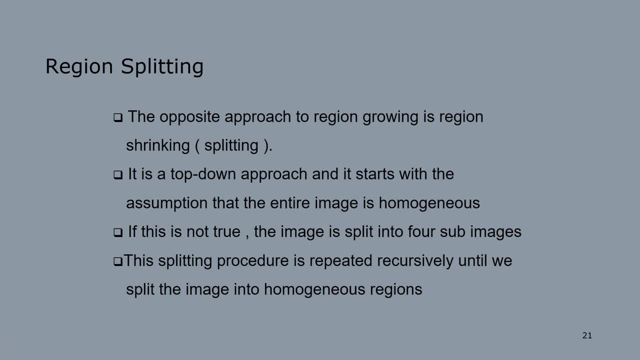 technique. The opposite approach to region growing is region shrinking, that is, the splitting. It is a top-down approach and it start with the assumption that entire image is homogeneous. So the assumption is the entire region is homogeneous and this approach is opposite to the region growing technique. 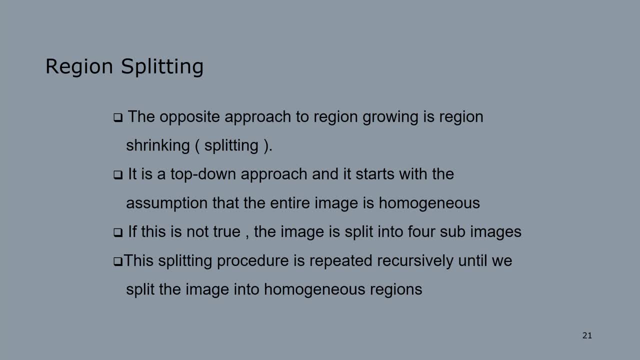 If this is not true, the image is split into 4 sub images. This splitting procedure is repeated recursively until we split the image into homogeneous regions. So this concept I am going to explain in the next slide. what is the meaning of this. So for this first, I am assuming that the entire image is homogeneous. 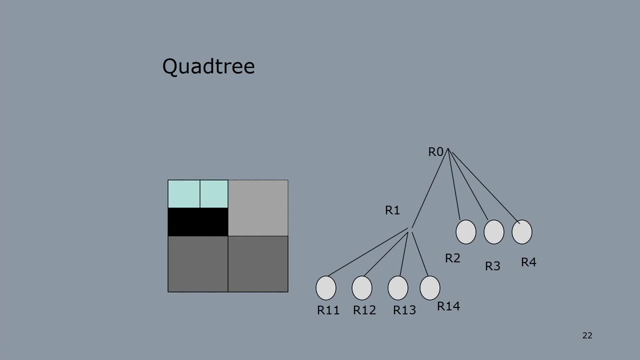 So in this case I am showing that entire image is homogeneous. If it is not true, the image is divided into 4 regions. So here you can see: this is my first region, this is my second region, this is my third region and this is the fourth region. 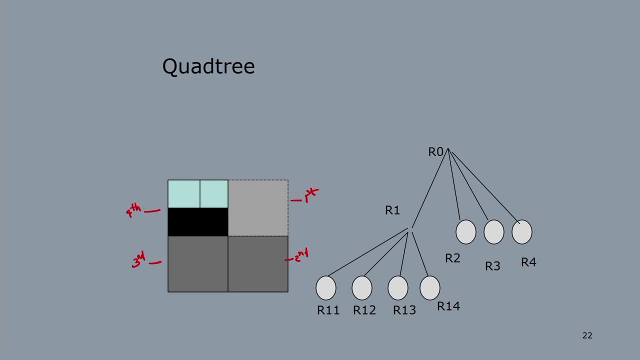 After this you can see in the first region that is homogeneous, So no need to do splitting. Second region: Second region is also homogeneous, So no need to do the splitting. The third region is also homogeneous, So no need to do the splitting. 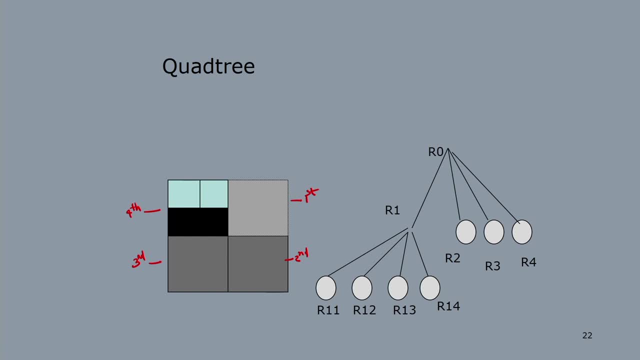 And if I consider the fourth region, that is not homogeneous. So what I have to do, I have to do the splitting. So I have to do the splitting, like this, into 4 regions And if you consider these 2 regions, if you consider these 2 regions, they are homogeneous. 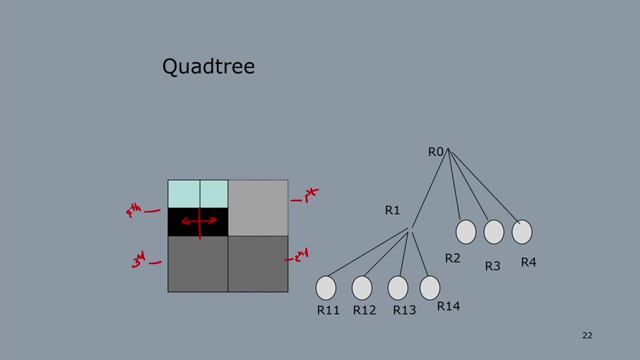 So these 2 can be merged together. See these 2 regions. these are homogeneous, that can be merged. So, corresponding to this procedure, you can see the quad tree. So this is the root of this. That is the region, that is the corresponding to the image. 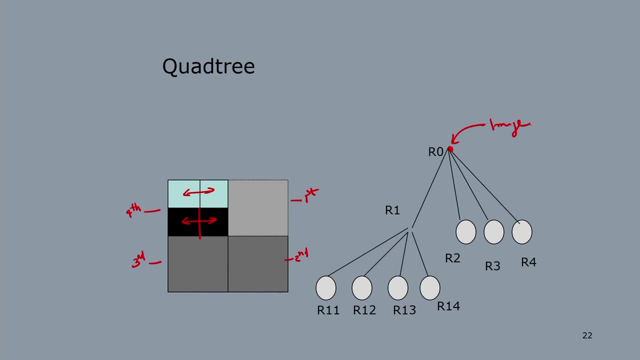 Corresponding to the entire image. this is the node R0.. The R0 is splitted into 4 regions. The regions are R1, R2, R3, R4.. Now R2 is homogeneous, So no need for splitting. 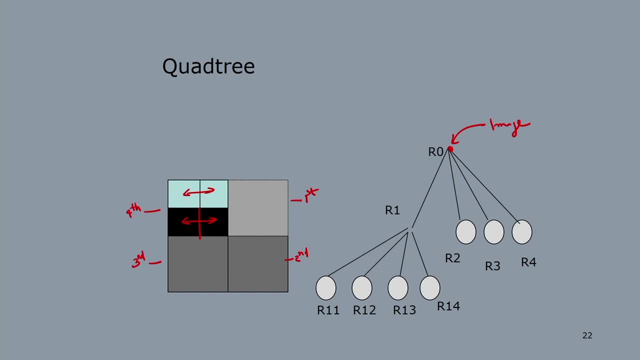 So this is R1.. R3 is homogeneous, So no need to do splitting. R4 is homogeneous, So no need to do splitting. But R1 is not homogeneous, So that is why it is divided into 4 regions. The regions are R11, R12, R13, R14. 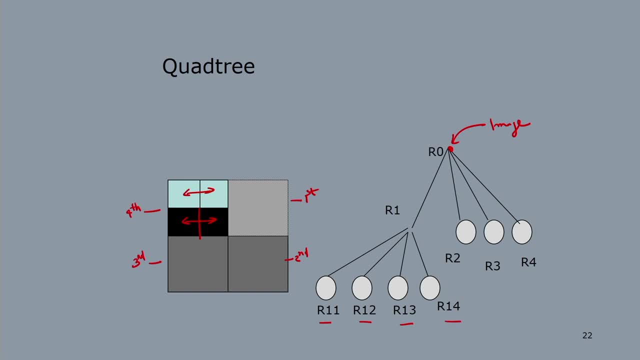 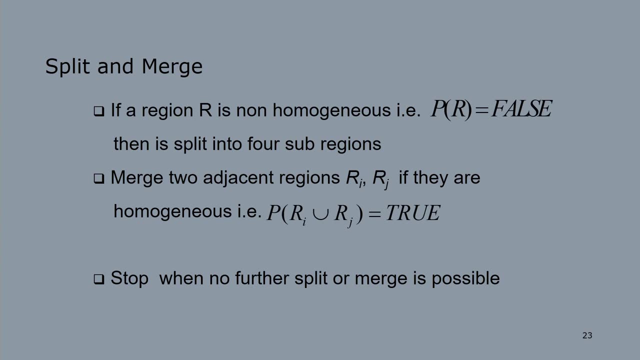 So this procedure I have to repeat. And also we have to do the merging, the splitting and merging. we have to do So for this the algorithm will be like this: If a region R is not homogeneous, then the predicate R will be false. 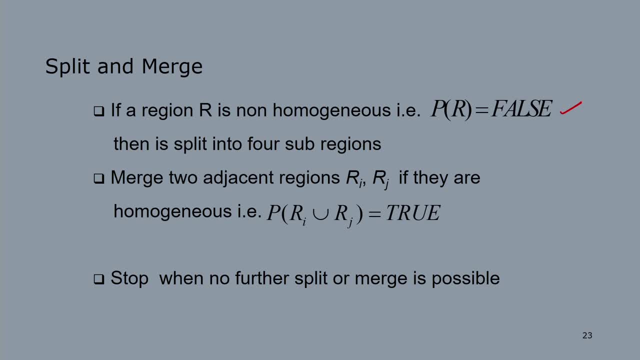 The predicate of the region is false, Then the split into 4 sub regions. If the region is not homogeneous- that is, the predicate of R- is false, Then the split the regions into 4 sub regions. After this, the merge 2 adjacent regions, Ri and Rj, if they are homogeneous. that is the. 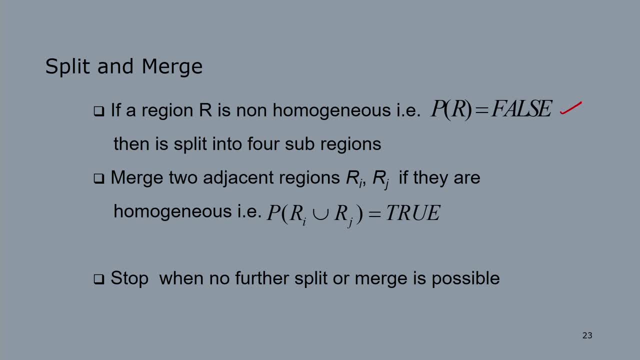 predicate of Ri union, Rj is equal to true, Then if it is homogeneous, I can do the merging Stop when no further splitting or merging is possible. So I have to repeat this And finally I will be getting the segmented image. 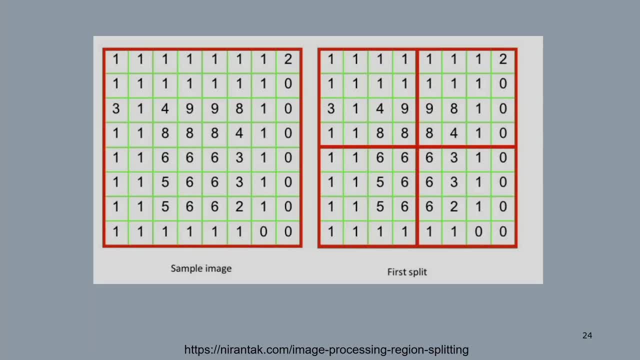 So here I have given one example. You can see, I am considering one image, the sample image, since it is not homogeneous, So I am dividing it into 4 regions. You can see 4 regions here: the first region, second region, third region and the fourth. 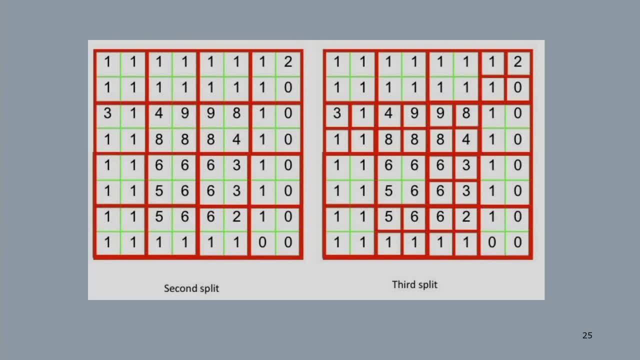 region. I am doing the splitting. Next slide. you can see the first region. what I have considered in my previous slide, that is not homogeneous, So that is why I am splitting into 4.. The 4 is the first region. second region, third region, fourth region, like this: 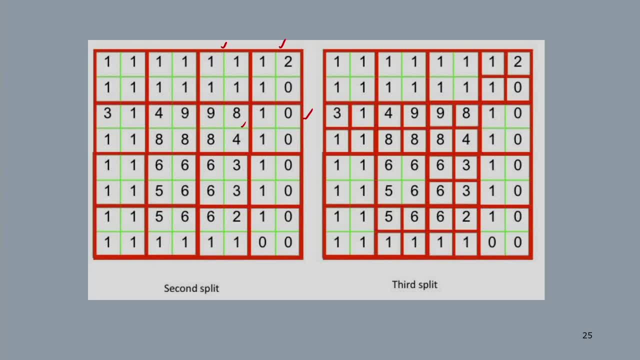 And similarly other regions also. that is not homogeneous, So that is why I am splitting it again. So this region, this region, this region and this region And similarly for other region also. since it is not homogeneous, so I am splitting into: 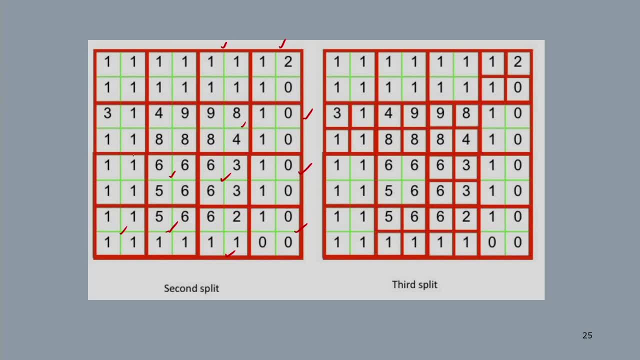 4 regions: this region, this region, this region and this region And, like this, the final. if I consider this region, final region, that is also not homogeneous. So that is why it is splitted into 4 regions In the third split, what I am considering. so this is homogeneous. 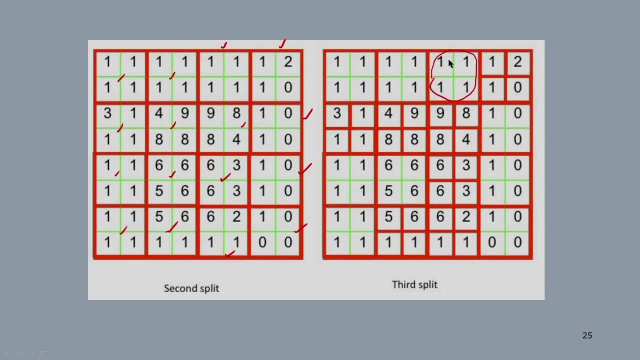 This portion is homogeneous. So then, in this case, no need for splitting. But this region is not homogeneous, So that is why I am doing the splitting, The splitting is done. So this region, I am doing the splitting- This region is homogeneous. 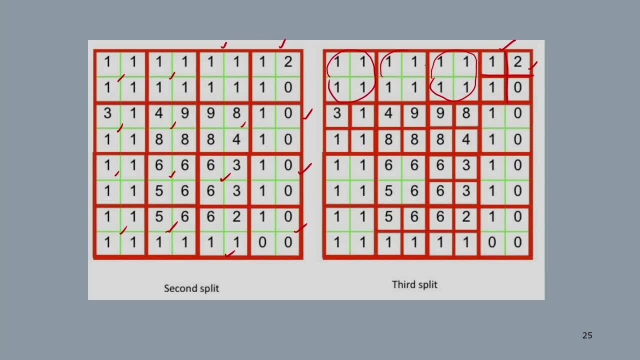 So that is why no need to split. This region is homogeneous, no need to split. But this region is not homogeneous. So that is why I am doing the splitting Like this I am doing: I am considering all the regions And I am doing the splitting. 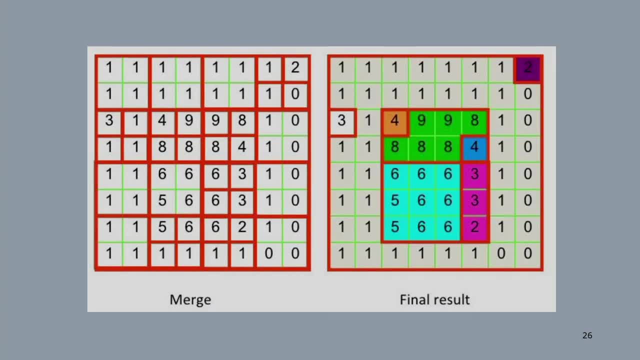 So this is the third split And after this I am doing the merging. So if you consider, this region can be merged with this, this can be merged with this, because this is homogeneous, and also this can be merged with this. But if you consider this portion, this, this two, two, I cannot merge. 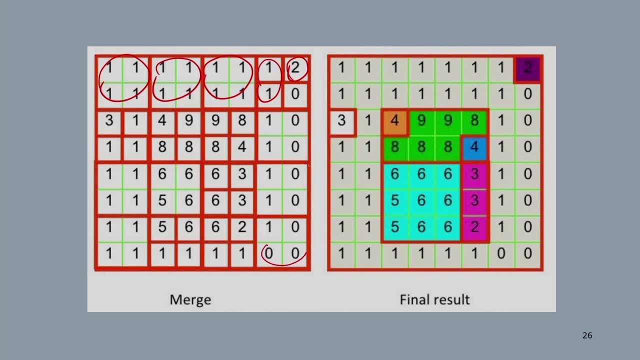 Similarly, if I consider this, all the 0, 0, 0''s that can be merged. Similarly, if I consider this this: 1 1, 1, 1, 1, this can be merged. 3 will be isolated. 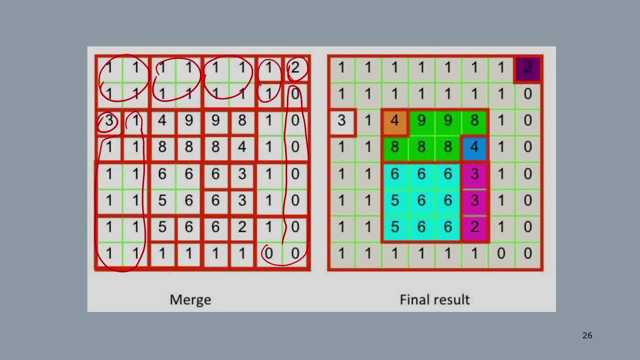 that I cannot merge Like this. I have to do the merging. So in the final result, what you will be getting: 2 will be isolated, 3 is isolated. that cannot be merged, and you can see the merge pixel. So you can see: 1, 1, 1. all these are merged. So these are merged. 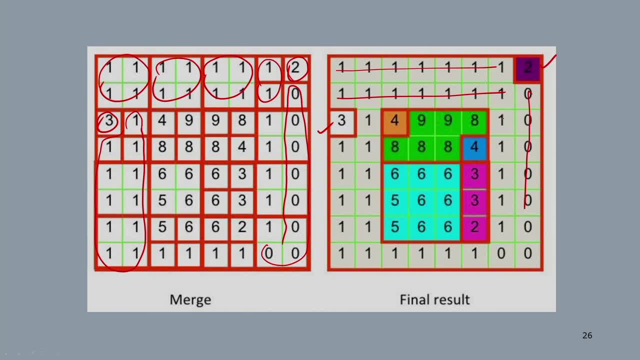 all these are merged 0s. all these are merged 1s. this is merged. this is merged. So I am just doing the merging. like the 6. I am doing the merging. the 5 is different, So I can. 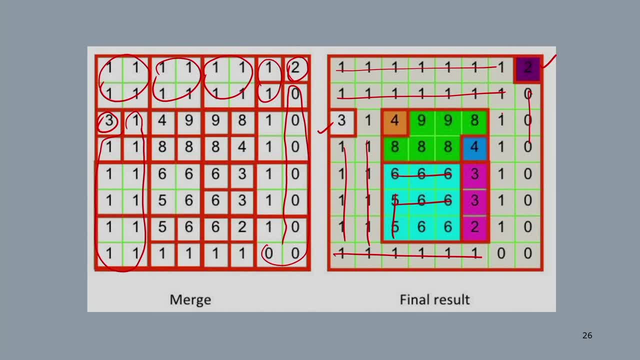 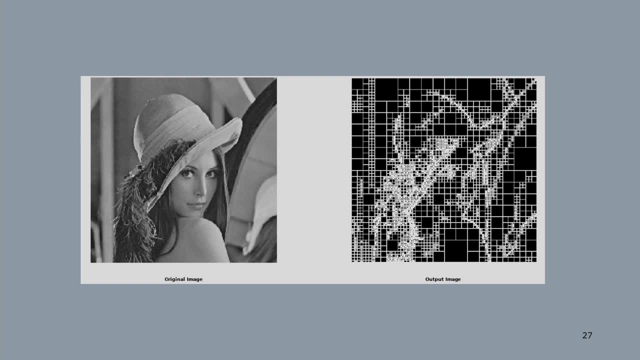 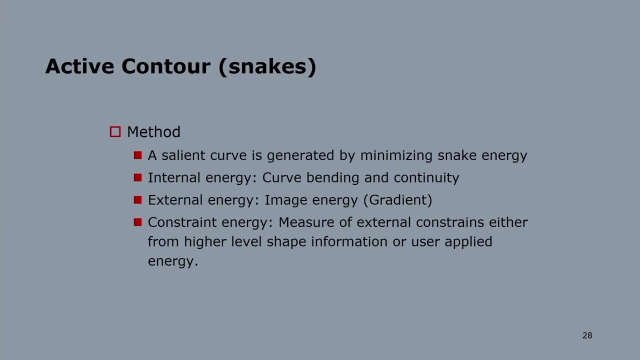 do the merging of the pixels, So I am getting the final results. So this is the technique of the splitting and the merging and, corresponding to this image- original image- I am applying this technique And you can see the output. Next, one important technique I am going to discuss that is active. 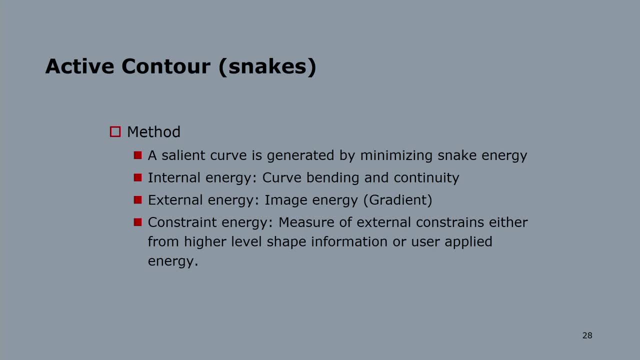 contour, base technique. So what we have to consider. Suppose, if I want to do the segmentation of an object, suppose one image is there and I have one object, suppose this object. So what I can consider, I can consider one contour, this contour, I can consider around this object. 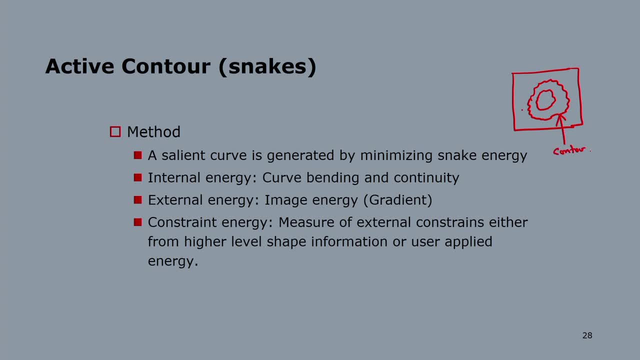 and this is called a contour around the object, And this is my object. and this contour, the or the snake, it is also called the snake. The snake has the internal energy that corresponds to curve, bending and the continuity. This snake has the external energy, that is, the image energy. and I am also considering some 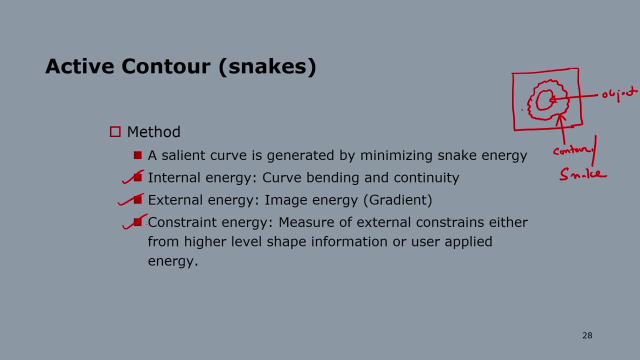 constraint energies, some constraints I am considering, That is, measure of external constraints, either from higher level shape information or from higher level shape information. So this is the energy that I am considering. So these energies, I am considering, one is the internal energy, external energy and the constraint energy. And in this case, what? 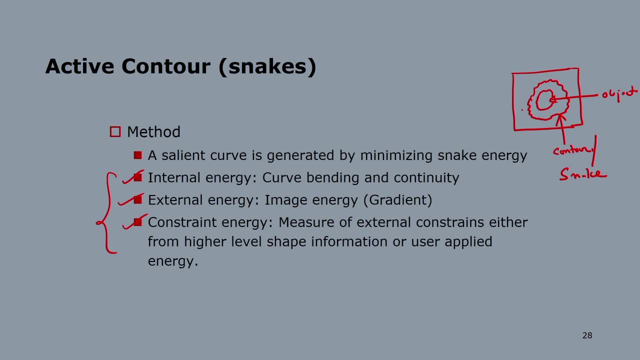 I have to do? I have to minimize this energy corresponding to the contour. When the energy is minimum, the contour touches the boundary of the objects. So my problem is I have to minimize this energy. So energy, the total energy, has three components: internal energy. 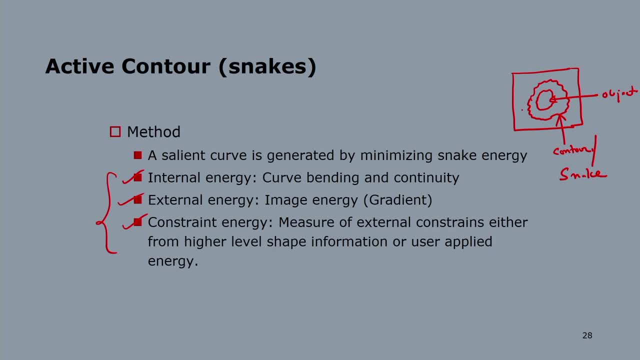 external energy and the constraint energy. So I have to minimize this energy. So energy, the total energy, has three components: internal energy and the constraint energy. So what I have to do, I have to minimize this energy and corresponding to this minimum energy. 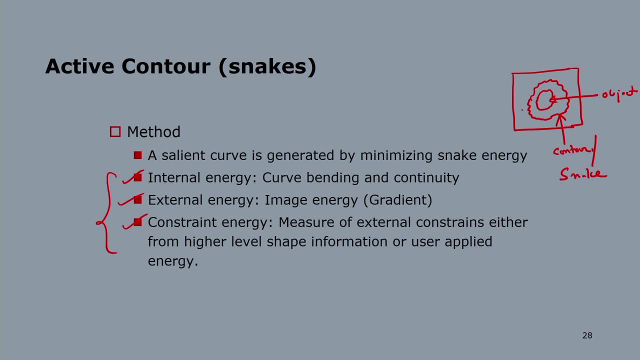 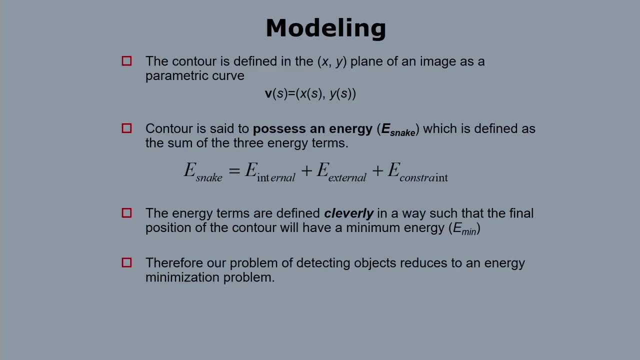 the contour touches the boundary of the object, that is the active contour. So how to define this energy? One is the internal energy, external energy and the constraint energy. So the contour is defined in the xy plane of an image as a parametric curve. So this is the definition. 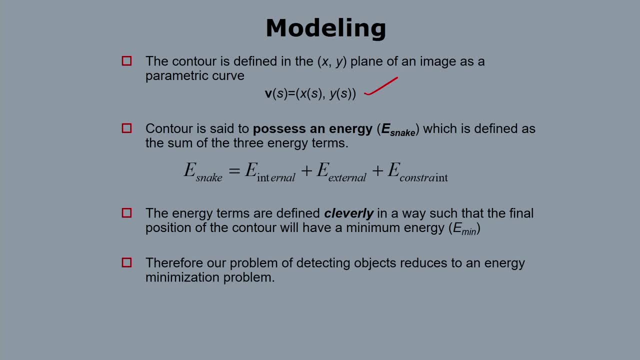 of the contour. The Vs is equal to xy, S, comma, ys and corresponding to this snake or the contour. I am considering these energies: One is the internal energy, one is the external energy, and also I am considering the constraints. So we have three energy terms Now. in this case, the energy terms are defined cleverly. 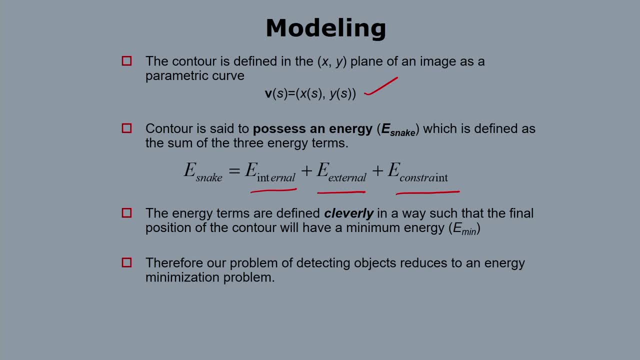 in such a way that the final position of the contour will have the minimum energy. So whenever the contour touches the boundary of the object, the energy will touch the boundary of the object, The energy will be minimum. So the problem is the energy minimization problem, The problem. 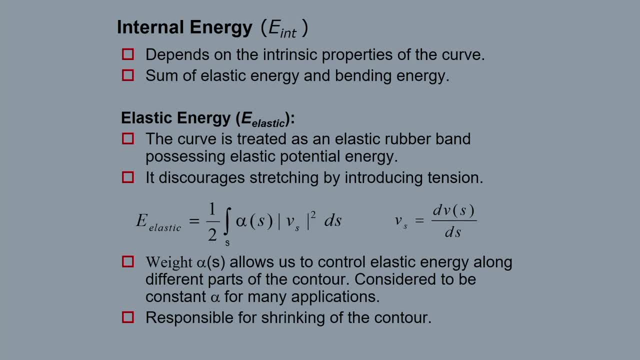 is the energy minimization problem. So how to define the internal energy? So internal energy depends on the intrinsic property of the curve, That is, the sum of the elastic energy and the bending energy. So what is the elastic energy? That means the internal. 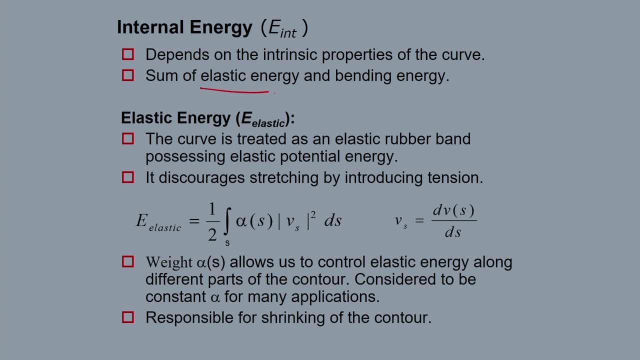 energy has two components: One is the elastic energy, another one is the bending energy. So what is the elastic energy? So what is the elastic energy? So what is the elastic energy? The curve is treated as an elastic rubber band possessing elastic potential. 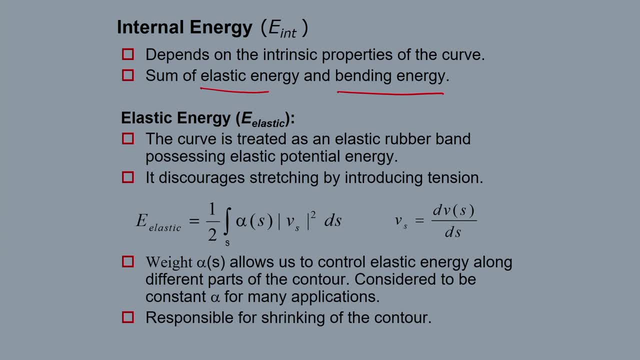 energy. So the curve is considered as an elastic rubber band possessing elastic potential energy. It discourages stressing by introducing tension. So the elastic energy can be defined like this: The weight is αs. That allows us to control the elastic energy который. 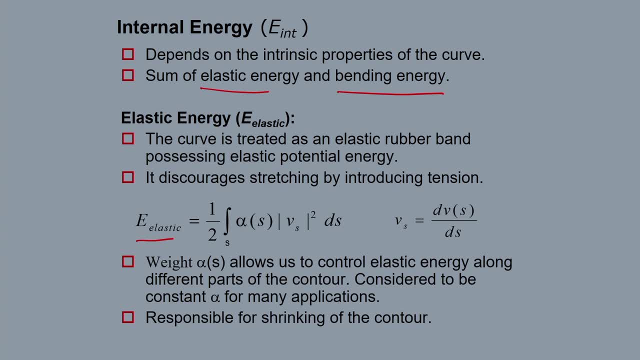 мы контрwny along different parts of the contour and for many applications this alpha s is considered as constant and this elastic energy is responsible, responsible for shrinking of the contour. So first, I am defining the elastic energy and you can see, so how to determine V s, V. 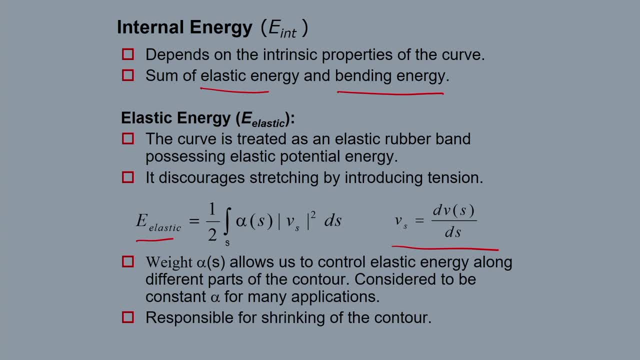 s is nothing, but I am just taking the gradient dV s divided by d s. that gradient I am considering So V s is defined like this. So first term is the elastic energy I am considering. The second term is the bending energy. You can see what is the bending energy, The snake. 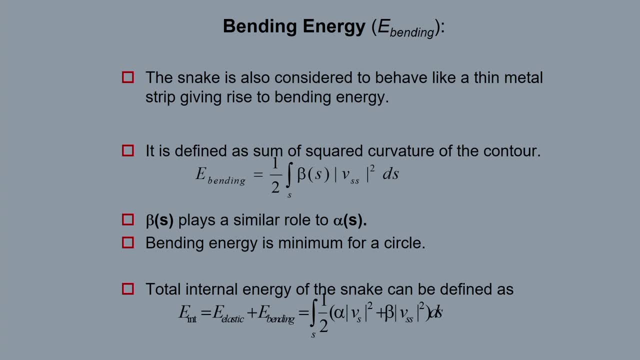 is also considered to behave like a thin metal strip, giving rise to bending energy, That this bending energy is obtained by this. It is defined as sum of squared curvature of the contour. That I can define the bending energy And V? s is very similar. 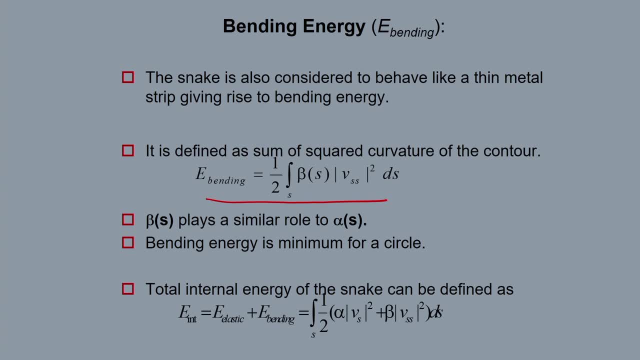 to alpha s. In many applications V s can be considered as constant. Bending energy is minimum for a circle, That is obvious. So bending energy for a circle will be minimum. So what will be my total energy? For total energy, I have to consider these two terms. 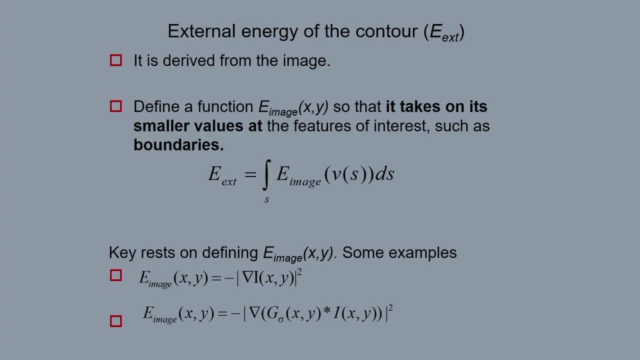 One is the elastic energy, another one is the bending energy. Next one is how to define the external energy of the contour. The external energy of the contour is derived from the image, So in this case you can see the definition of the external energy: E. external is equal. 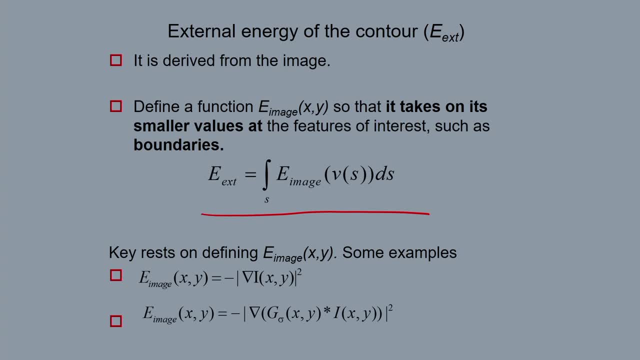 to integration. I am taking for the variable s, E image into V, s, d s. So what is E image? E image is nothing but it is the energy obtained from the image. So define a function E image so that it takes on its smaller value as the feature of the interest. 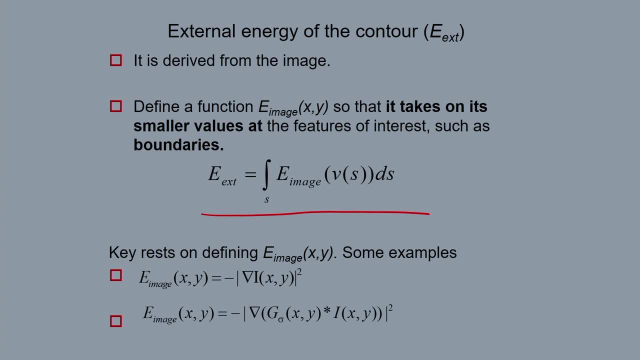 Such as boundaries. So that means I have to define the function E image so that it takes on its smaller value at the features of interest such as boundaries, So at the boundaries we have to consider. So this is the definition of the external energy and that is derived. 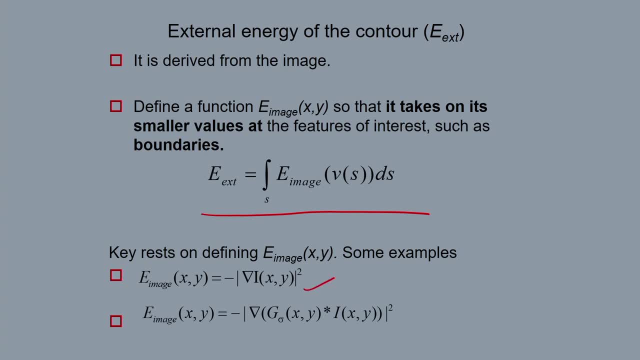 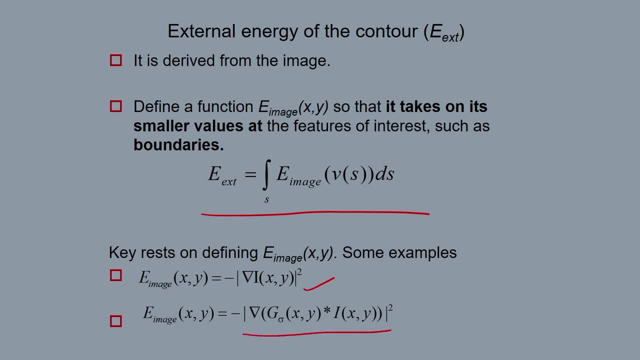 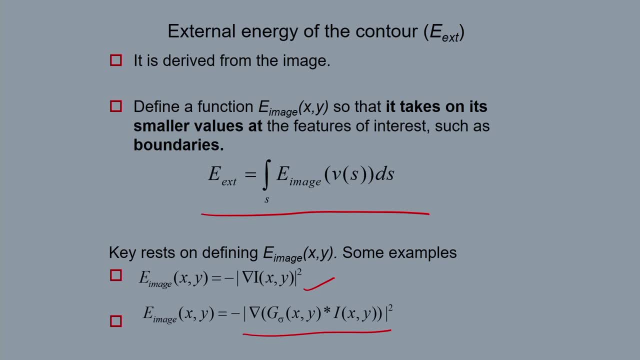 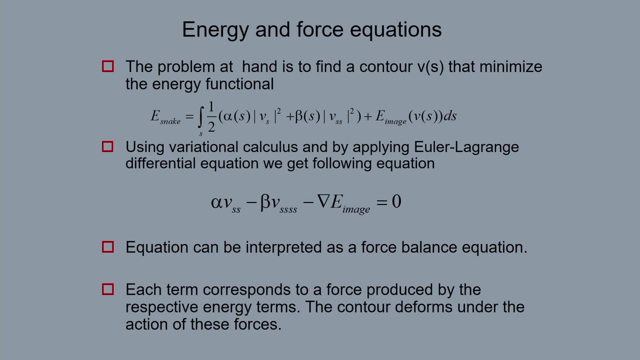 the gradient And from this you can determine the image energy. So, finally, the problem at the hand is to find the contour V s that minimise the energy functional. So the problem is, we have to minimise the energy. So energy- here I am considering the 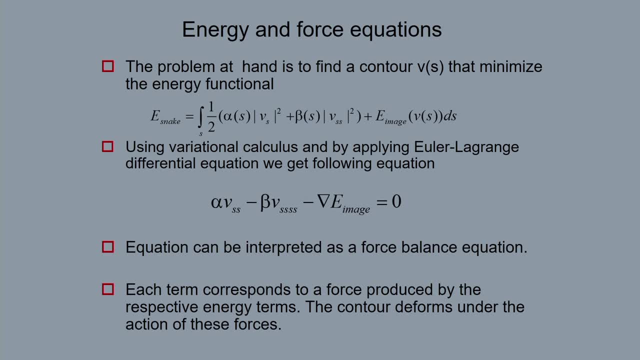 the internal energy and the external energy. The external energy is derived from the image itself And in this case we have to apply the Euler-Lagrange differential equation. So this Euler-Lagrange differential equation I have to apply and I will be getting this. 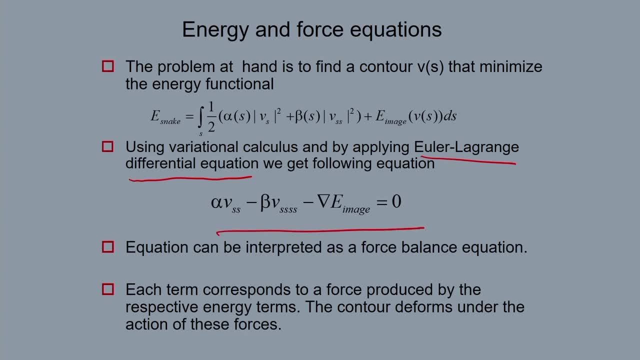 the energy minimization problem. So this equation can be interpreted as a force balance equation. Each term corresponds to a force produced by the respective energy terms. The contour deforms under the action of these forces, And whenever the contour touches the boundary of the objects, the energy will be minimum. 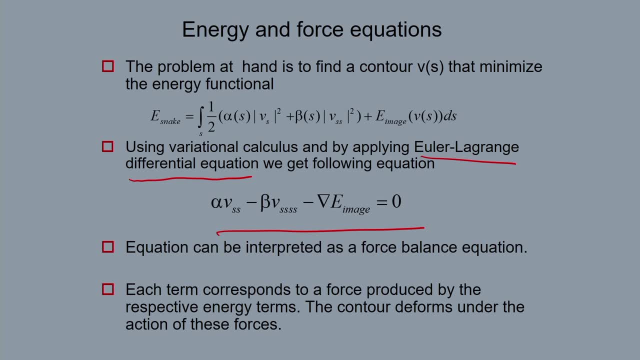 So this is the case. So the problem is the energy minimization problem, And for this we have considered the internal energy, external energy, And in this expression I have not considered the constraints, So only I have shown the two energy. 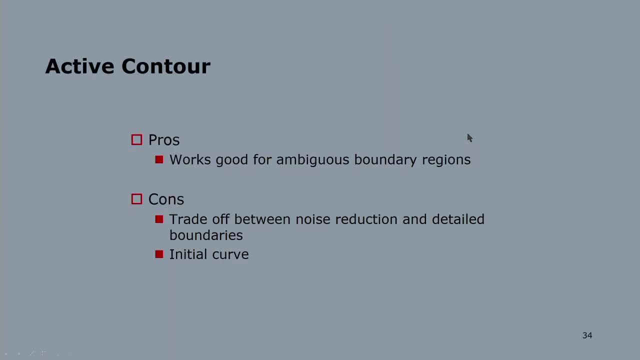 One is the internal energy, another one is the external energy. So what are the advantages of this technique? So it works good for ambiguous boundary regions, But the problem is how to define the initial curve. That is also the problem of this method. 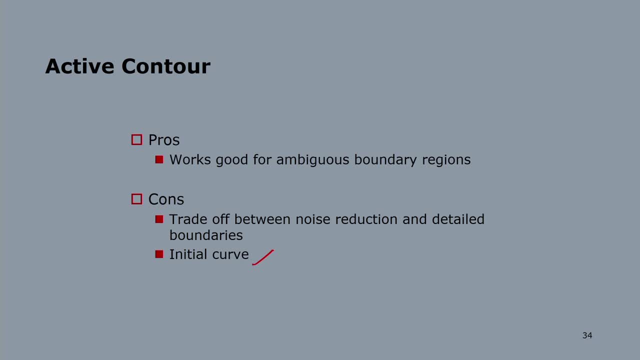 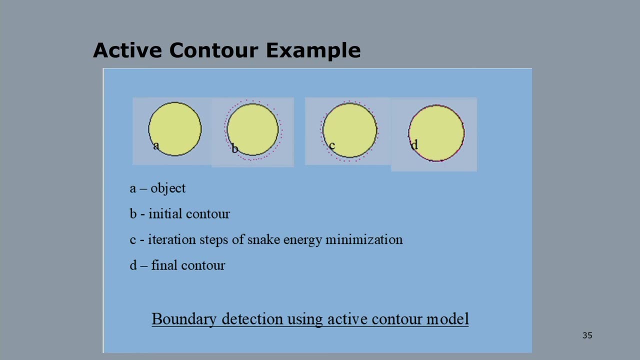 And also the trade-off between noise reduction and the detail boundaries. So I can give some examples of the active contours. You can see A is the object And initially I have to define the contour. So B is the contour here. If you see the dotted line, that is the contour. 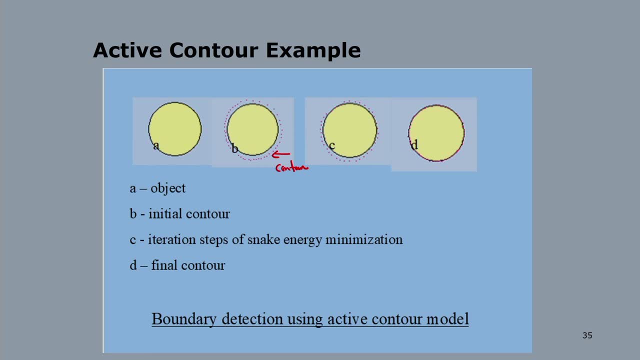 And after this, what I have to consider? I have to consider the energy, The energy of the contour, that is, the internal energy and the external energy. And after this, with each and every iteration, I have to minimize the energy. That is the snake: energy minimization I have to do. 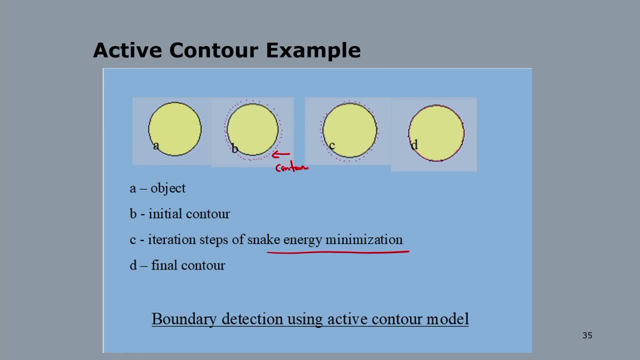 And whenever the contour touches the boundary of the object, the energy will be minimum And that corresponds to the final contour. That D is the final contour And that is the segmented object I will be getting. So the segmented object I will be getting when the contour touches the boundary of the 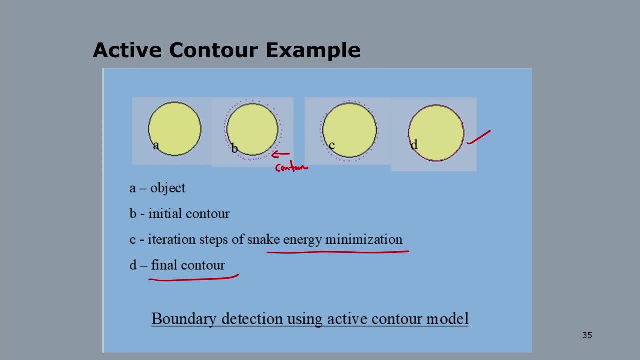 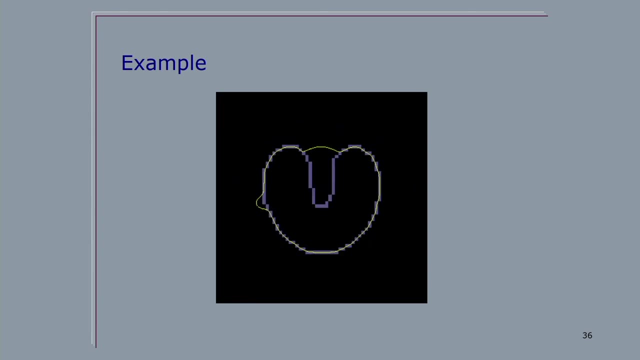 object. This is the boundary detection using active contour model, And here I have given another example. You can see the initial contour And after this I am doing the energy minimization. Energy is nothing but the internal energy and the external energy. 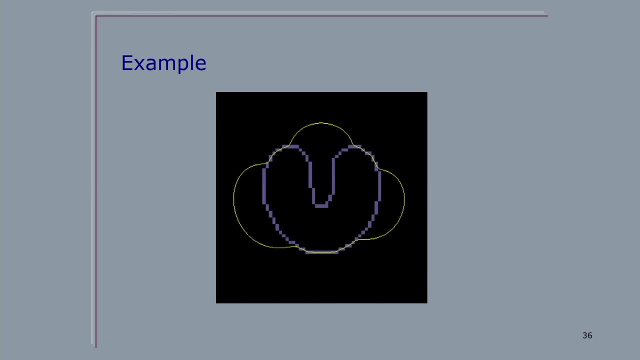 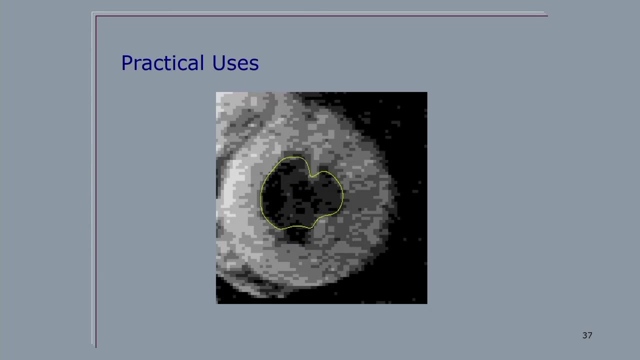 And whenever the contour touches the boundary of the object, the energy will be minimum. Another example I can show this is the segmentation of the mammogram, And I am defining the contour. See, with each and every iteration, the contour just touches the boundary of the objects. 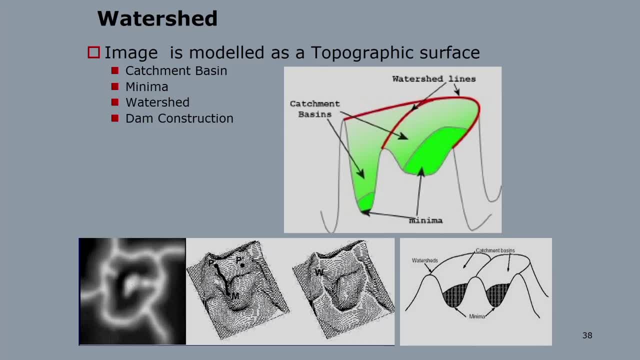 So I can do the segmentation by using active contour. The another popular technique is the image segmentation, That is, the topographic based segmentation technique, That is the watershed algorithm. So in this case the image is modeled as a topographic surface. So here in this figure- the first figure you can see- I am showing the topographic surface. 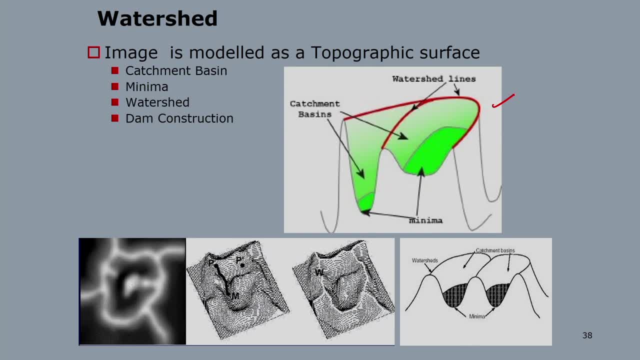 corresponding to the surface And corresponding to this topographic surface. you can see two castman basins. You can see two castman basins are available And corresponding to these two castman basins, I have the minima. this is one minima for 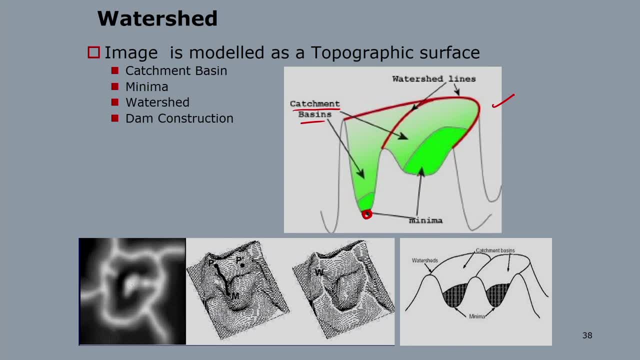 corresponding to the first castman basin, and you have another minima corresponding to the second castman basin, And between these two castman basins I have the watershed lines. you can see the watershed lines, the watershed lines. So that means the main concept is: what is the catchment basin, what 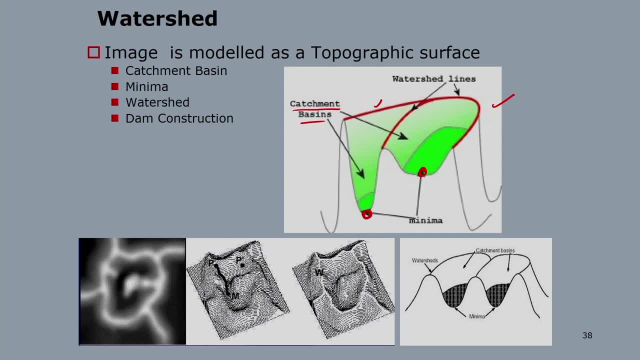 is the local minima and what is the watershed lines. and I will discuss about the dam construction, how to construct the dam. So that concept I am going to discuss. So the main concept is the image is modeled as a topographic surface, So corresponding to the figure 1, you can. 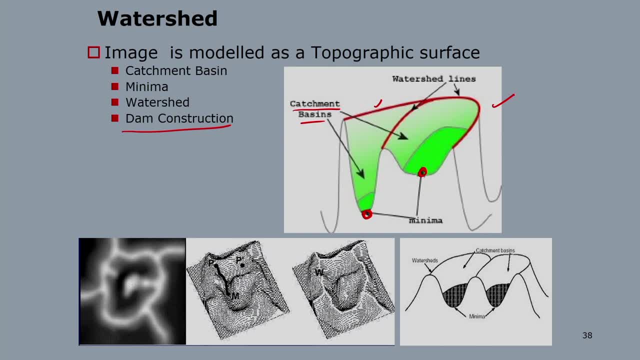 see two minima and I have considered two catchment basins and corresponding watershed lines. So corresponding to the this image, grayscale image- you can see the catchment basins, maybe the catchment basin here, and in this case I am considering a topographic. 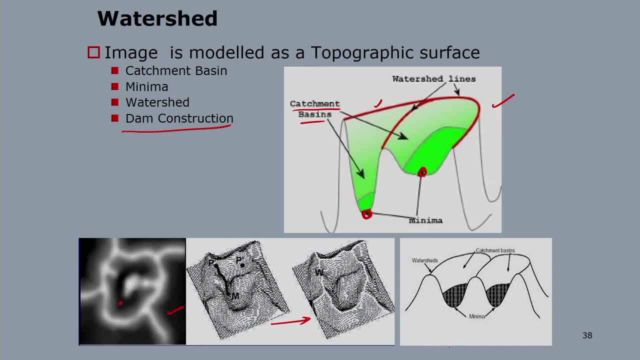 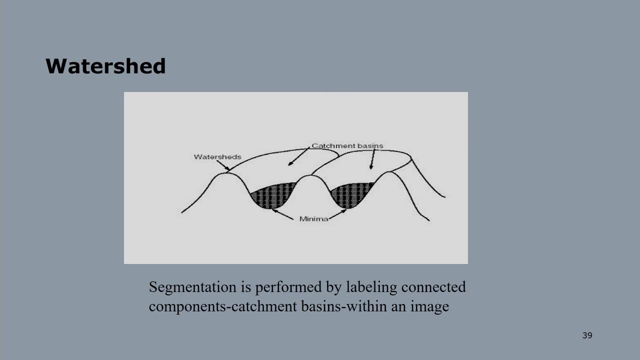 surface. This is the topographic surface and, corresponding to this topographic surface, you can see two minimas corresponding to two catchment basins, and again you can see the watershed lines. So in case of the watershed segmentation, segmentation, the segmentation is performed by labeling connected components, catchment. 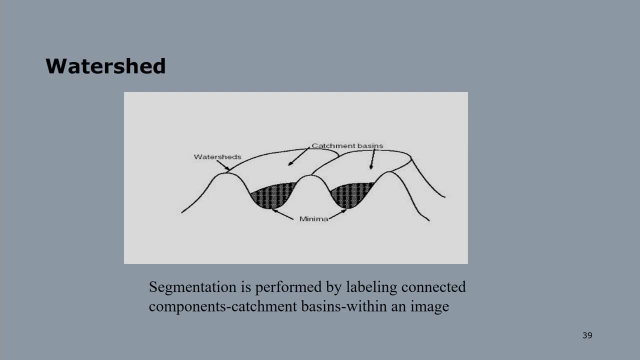 basins within an image. So in this case, what I have to consider, suppose corresponding to this, the first catchment basin, this is the minimum. corresponding to the second catchment basin, this is the minimum. Now the objective is to find the watershed lines between the catchment basins. 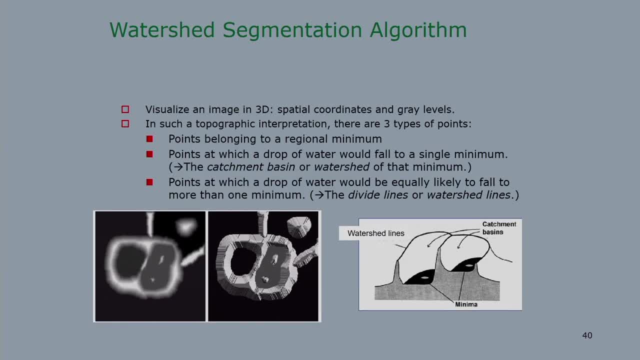 So that concept I will explain in my next slide. Here you can see, So visualize an image in 3D spatial coordinates and the gray levels I have to consider In SASE topographic interpretations. there are three types of points: points belonging: 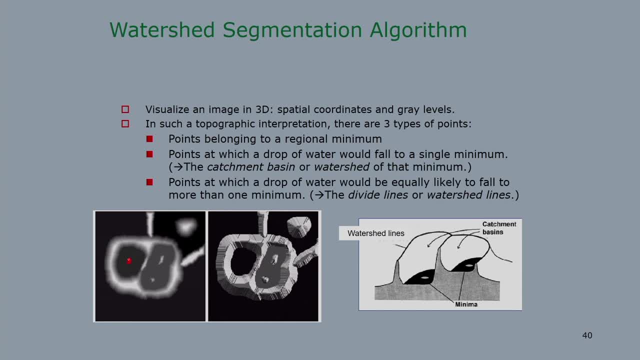 to a regional minima. So here, in this case you can see, suppose this point has a regional minima. So in the second figure also you can see we have the regional minima. The second point is point at which a drop of water would fall to a single minima. 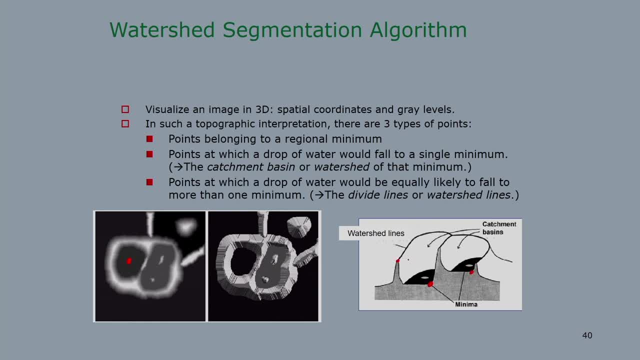 Suppose, in this case, if I put some water here, suppose corresponding to this, the drop of water would fall to a single minima, Single minima. suppose drop of water it falls into this minima Point at which a drop of water would fall to a single minima that I am considering. 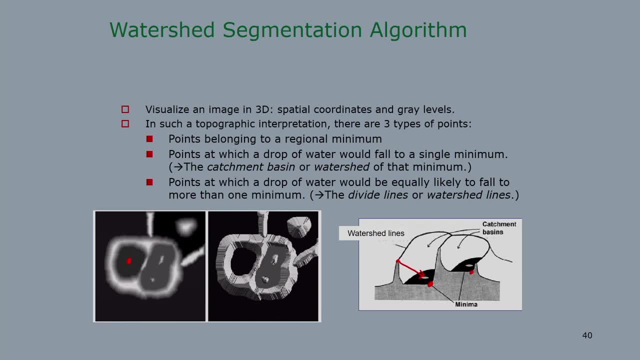 That is the catchment basin or the watershed of that minima. So if corresponding to this minima, if I put some water at this point, It would drop to this single minima. Third point is point at which a drop of water would be equally likely to fall into more. 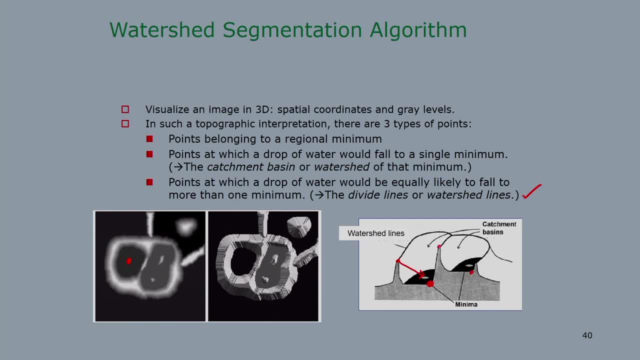 than one minima. Suppose, if I put a drop of water here, This drop of water would be equally likely to fall to more than one minima. So this drop of water may fall to this minima or may fall to this minima. 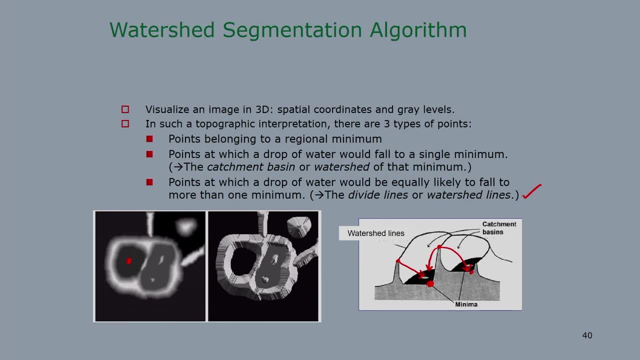 So you can see we have three types of points: Points belonging to a regional minima. That already I have shown the regional minima Point, as which a drop of water would fall to a single minima. So I am considering this point. 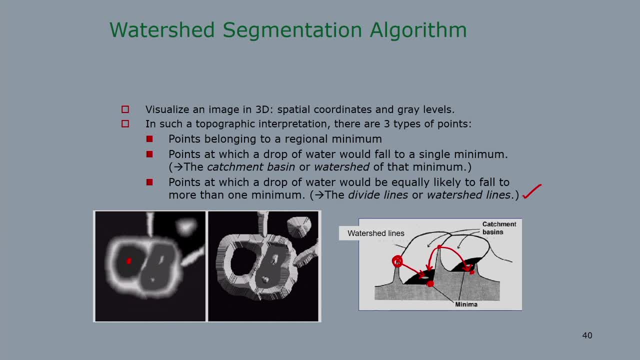 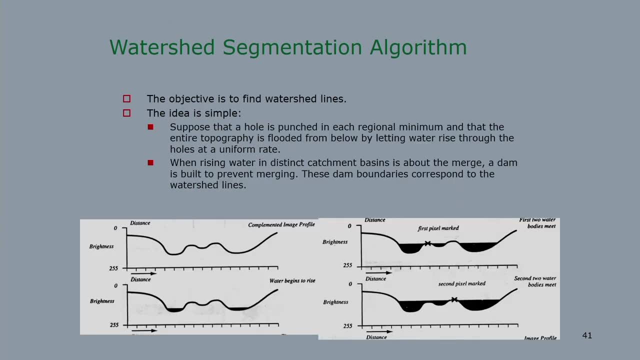 And points at which the drop of water would equally likely to fall to more than one minima, So that I am considering this one. So idea is how to determine the watershed lines. So objective is to find the watershed lines. So idea is very simple. 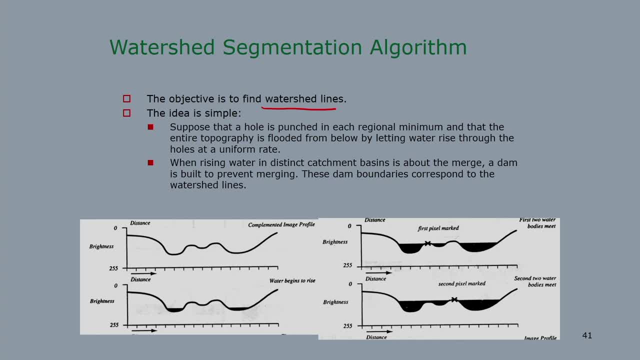 Suppose, in this case I have shown in this figure the brightness profile with respect to the distance. Now what I am considering, suppose in this brightness profile of the image, a hole is punch in the east of the regional minima. So in this case, this is my regional minima, this is my regional minima, this is my regional 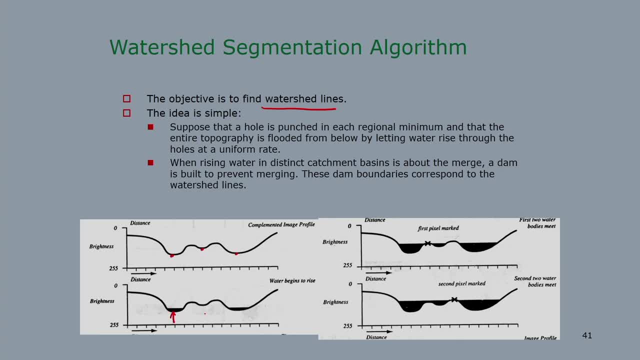 minima like this. So a hole is punch here, maybe here. maybe here the hole is punch in east regional minima that the entire topography is flooded from the below. So it is flooded from the below. Okay, So by letting water rise through the holes at a uniform rate, 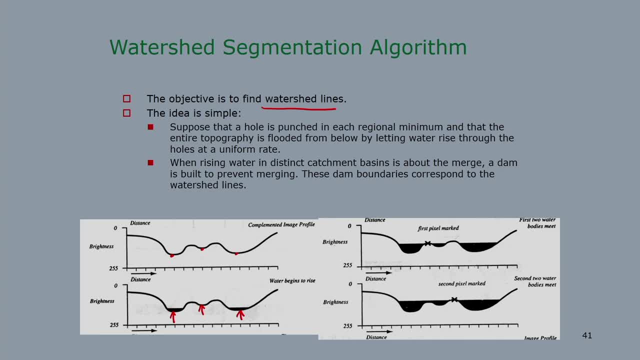 So just I am doing the flooding. So how to do the flooding? The flooded from below, by letting water rise through the holes at a uniform rate. So for this I am considering the holes like this: this is one hole, another hole like this: 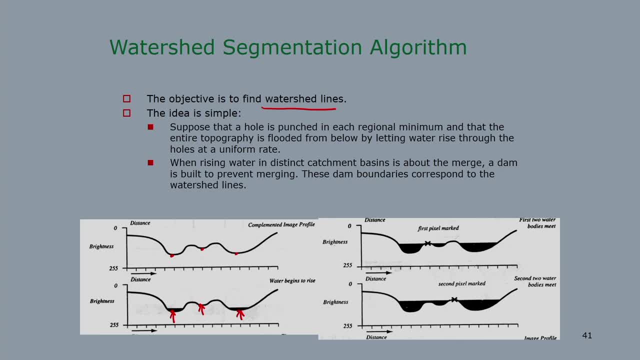 So water is rising now. So, whenever water is rising, what will happen at a particular time or particular point this water is about to merge to, this water about to merge, When rising water in distinct catchment basins is about to merge, So that how to prevent this flooding? then a dam is built to prevent merging. 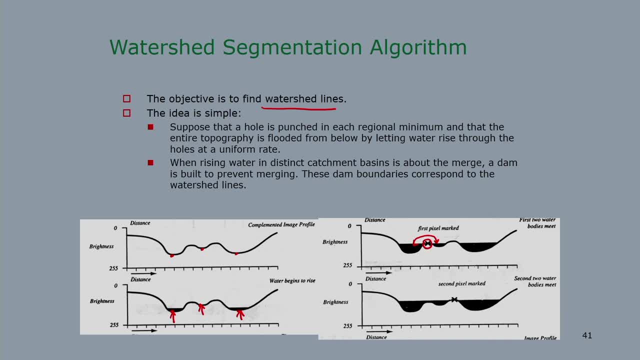 So that is why I am making a dam here, So that water cannot flow from one catchment basin to another catchment basin. So that is why I am constructing a dam, So that the water cannot merge, So that the water cannot merge from one region to another region. 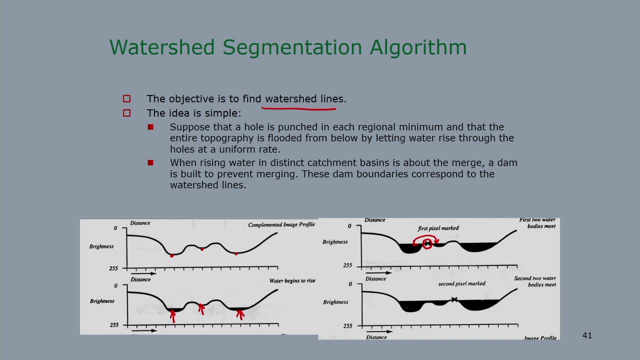 This dam boundaries corresponds to the watershed lines, Similarly corresponding to these two regions. this is one region and another region is this: The flooding is going on. What I am doing? flooding from below by letting water rise through the holes at a uniform rate. 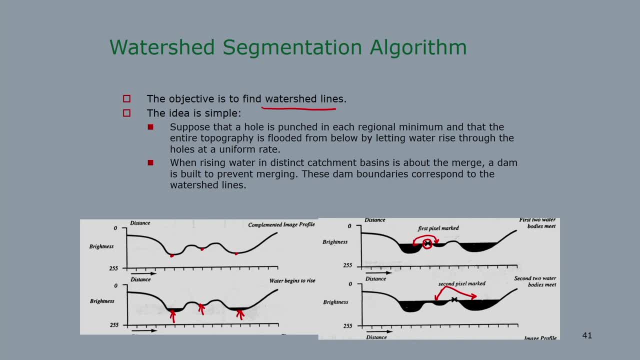 So what will happen? to prevent merging of water from this, both the regions- I have to construct a dam, So dam construction is going on like this. This dam boundaries corresponds to the watershed lines, So that means the objective is to find the watershed lines. 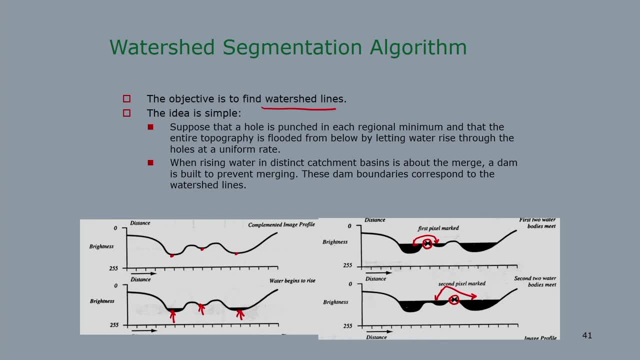 So that is called a dam construction. Dam construction is done so that the merging is not possible. That is, water is rising from the bottom and I want to prevent water coming from one region to another region. So for this a dam is constructed So that water cannot merge. 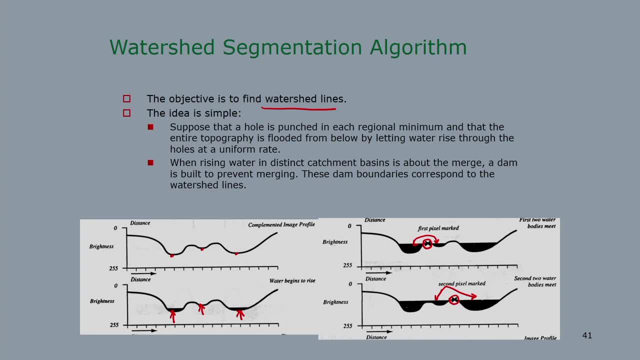 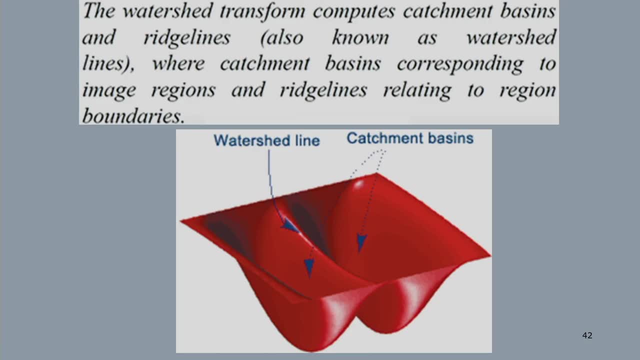 So I have to merge from one region to another region and I have to do the dam construction like this, and this dam boundaries corresponds to the watershed lines. So this concept again I am showing here. I have shown in this figure the catchment basins. I have shown and also I have shown 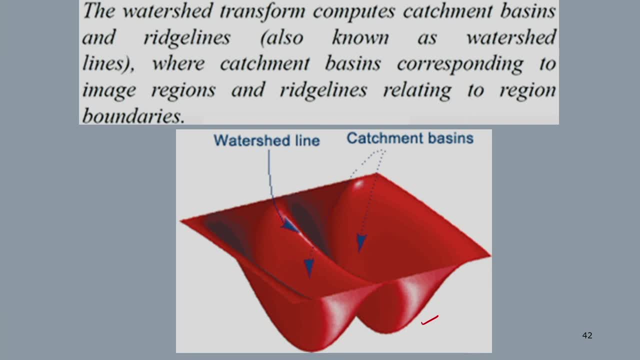 the watershed lines. So objective is to determine the watershed lines, The watershed test from compute catchment basins and the ridge lines. these ridge lines are also known as watershed lines, Where the catchment basins corresponds to the image regions and the ridge lines corresponds. 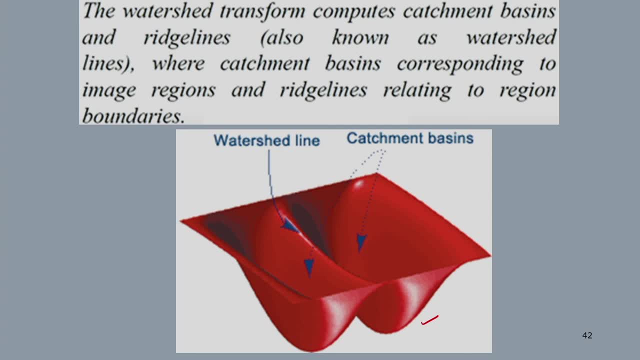 to the region boundaries. So that means I have to identify the watershed lines based on this principle- And in this case the catchment basins- corresponds to the image region. So this is the image region. like this, this is the image region, and if I consider the 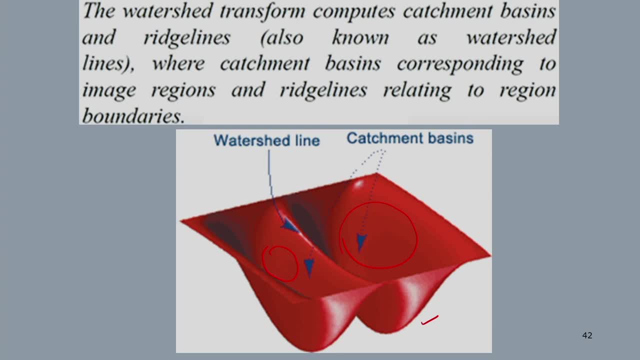 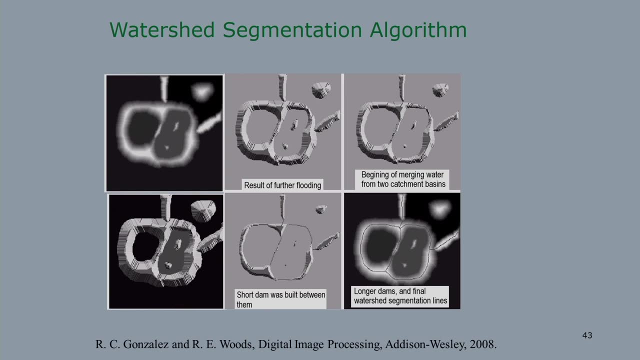 ridge line. This is the watershed line that corresponds to the region boundaries. So if you consider this one, this is the region boundaries. So in this example, I have shown how to construct the dam. So you can see the flooding is going on. result of the flooding. 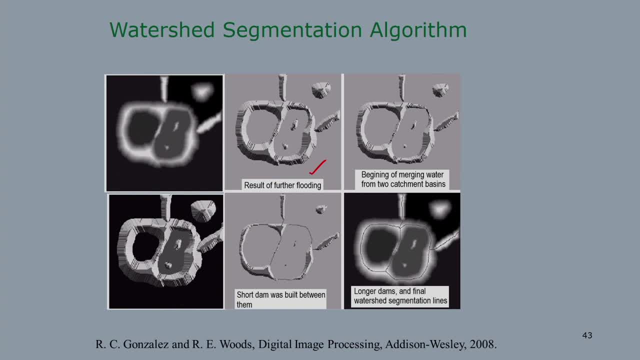 And for this the water is about to merge from two catchment basins. So the water is about to merge, you can see. So for this, a short dam is constructed so that the flooding is not possible from one region to another region. So I am constructing a dam so that water cannot merge from one region to another region. 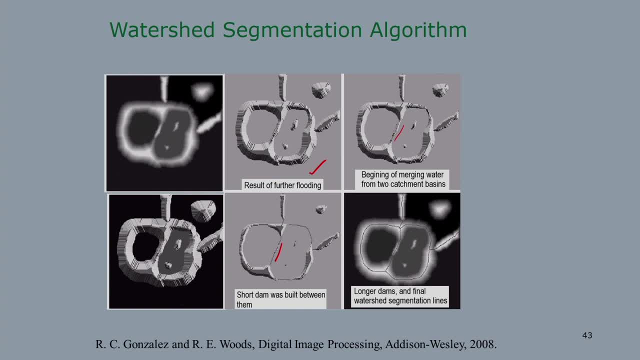 And finally, you can see, I am constructing a longer dam. that is the watershed lines, So that water cannot merge from one region to another region. Water cannot flow from one region to another region. That is, I am determining the watershed lines. So you can see the final results I have shown. 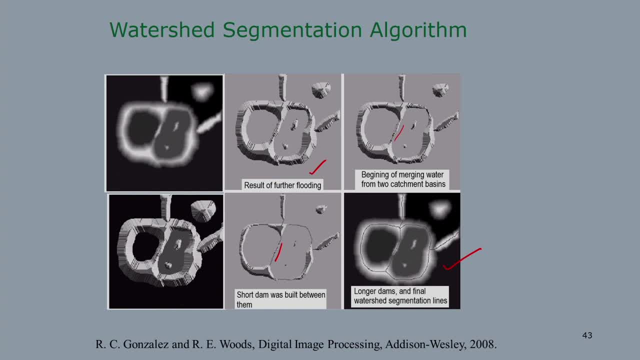 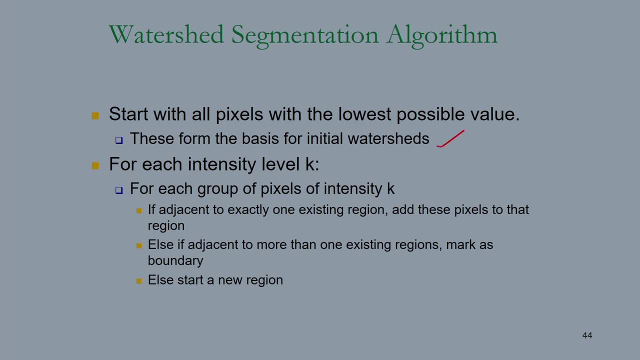 The longer dams are constructed and that is the final watershed segmentation line. So algorithm will be like this: whatever I have explained here start with all pixels with the lowest possible value. this from the basis for initial watersheds. Now for each intensity level: k for each group of pixel of intensity, k if adjacent to exactly. 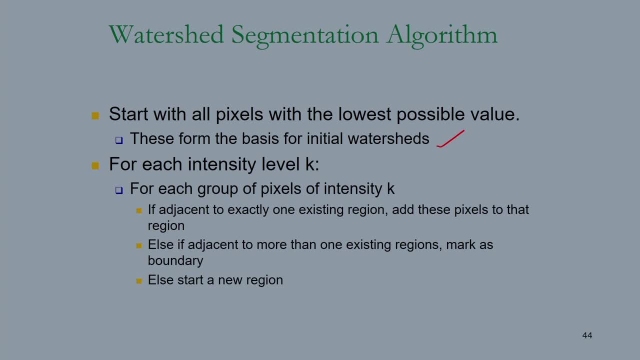 one existing region, add these pixels to that region. else, if adjacent to more than one existing regions, mark as boundary. That means I am determining the watershed lines, else start a new region. So that is the concept. That means I have to find the watershed lines. 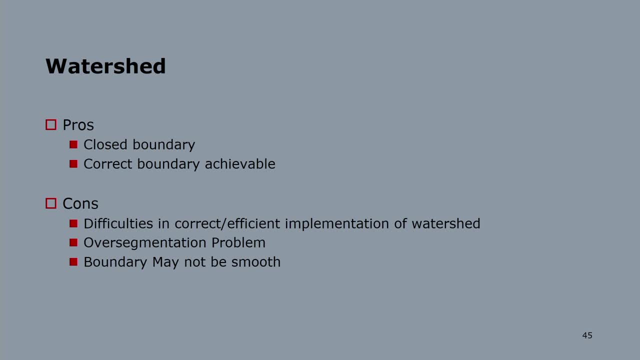 So what are the advantages of the watershed segmentation? Close boundary is obtained and correct boundary achievable, And one main problem is over segmentation problem. So what is the over segmentation problem? Suppose, if I want to do the segmentation of these objects, this object suppose what I 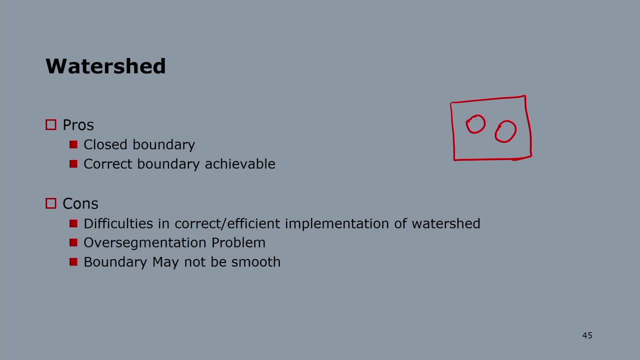 have to determine. I have to separate the objects from the background. So this is my object and I have to separate it from the background. But what is the over segmentation? Because of the over segmentation, what happened? Objects being segmented from the background are themselves segmented into sub components. 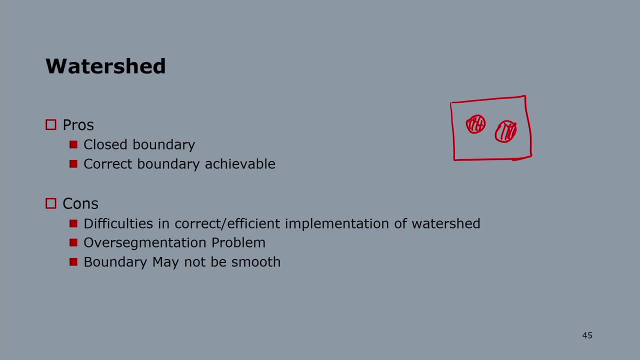 So that means this will be segmented out. So that means it is again segmented into sub components. That is not desired. So over segmentation is a big problem in watershed algorithm. The over segmentation means Again I am repeating- the objects being segmented from the background are themselves segmented. 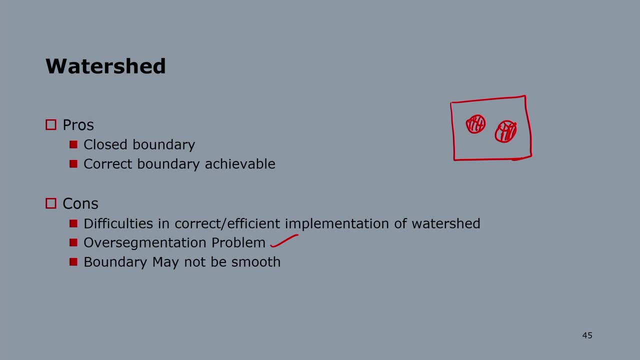 into sub components. That is the over segmentation. So this over segmentation is a problem And what is the approach? The solution is: I have to do the filtering, and by filtering I can remove weak edges. That is one method. The over segmentation is a big problem in watershed algorithm. 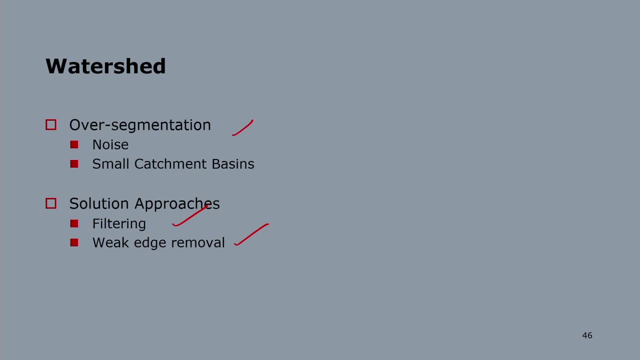 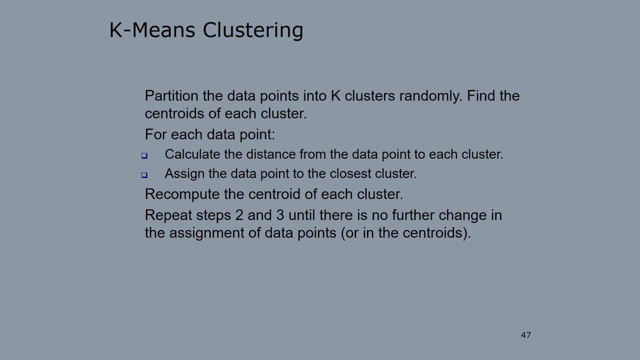 So that I can consider by filtering. So by filtering I can remove the weak edges. And finally I want to discuss the algorithm. that algorithm is the k-means clustering. So what is the k-means clustering Partition, the data points into k number of clusters randomly. 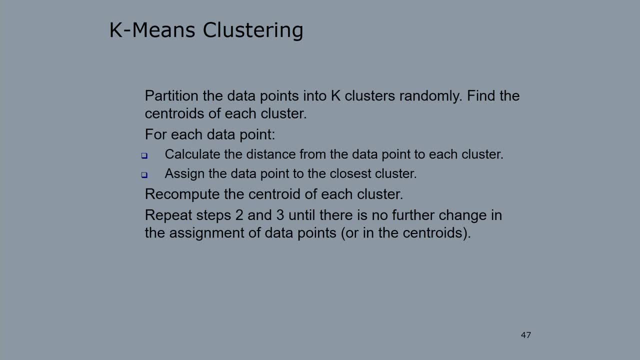 Find the centroid for each cluster. I have to find the centroid for each cluster For each data point. calculate the distance from the data point to each other cluster. Assign the data point to the closest cluster. Recompute the centroid for each cluster. 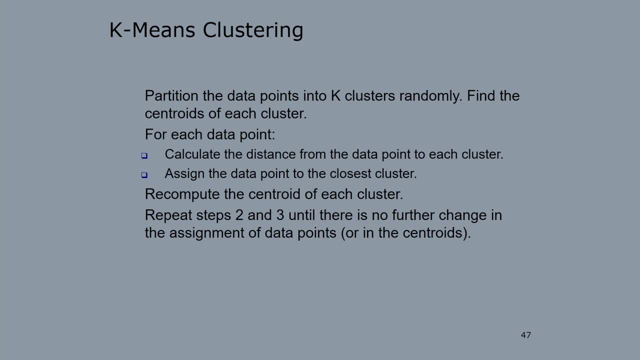 Recompute the centroid for each cluster, Repeat step 2 and 3 until there is no further change in the assignment of the data points or in the centroids. Now I am going to discuss about the k-means clustering. So what is k-means clustering? 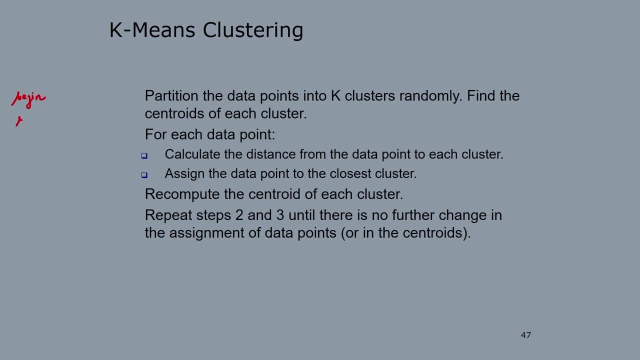 So I will explain, So begin. So first I have to initialize n number of data points, or maybe the samples. c number of clusters And corresponding to the c number of clusters, I have the centroid. The centroid are mu 1, mu 2, up to mu c. c number of centroid. 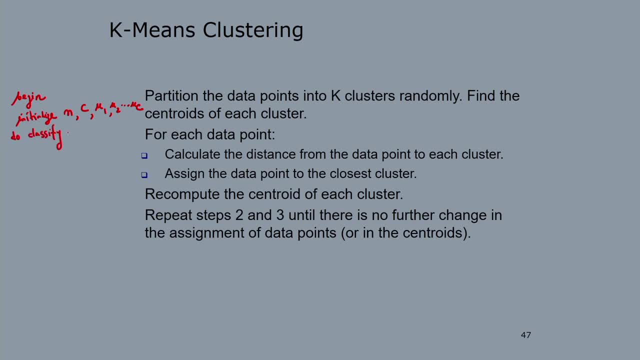 After this, what we have to do Do classify n samples according to nearest mu i. So I have to do the classification n samples according to nearest mu i, And after this, again I have to recompute, Recompute the centroid. 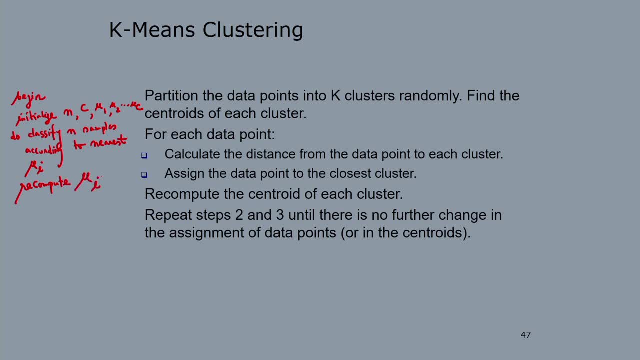 Do classify n samples according to nearest mu i And after this again I have to recompute The centroid. the centroid is mu i. Until no change of mu i, What will be my return value? Return mu 1, mu 2 like this: 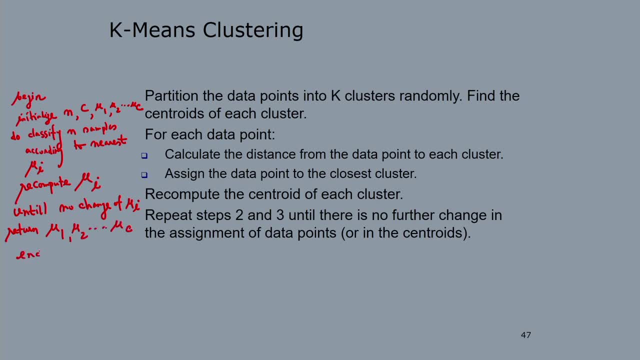 I have c number of centroid in there. So this is the algorithm for the k-means clustering. I have to initialize the c number of centroid. So I am considering c number of clusters, suppose. So I have to initialize. initialize c number of centroids. n means the number of samples. Do classify n samples. 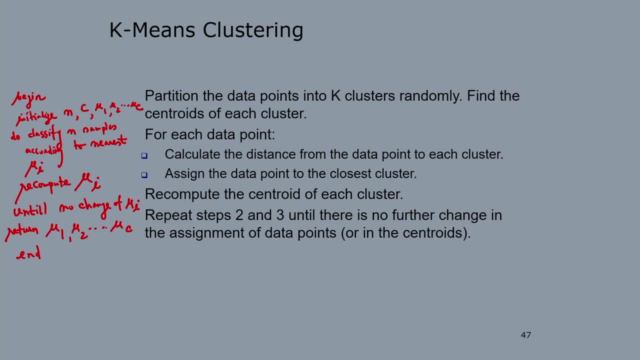 according to nearest of mu i. After this I have to recompute mu i until no change of the centroid. the centroid is mu i And finally I will be getting the centroids of the cluster, mu 1,, mu 2,, mu c- like this. That means this procedure is the clustering of the data points. 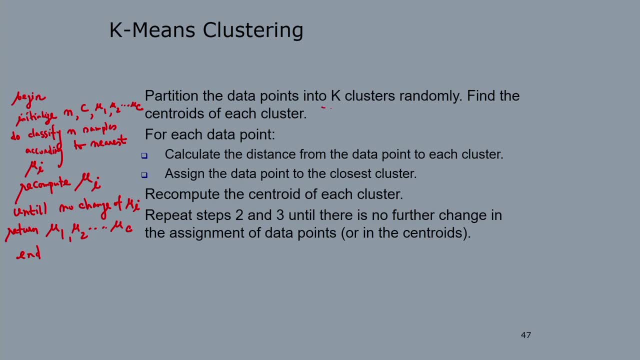 So this algorithm already I have written. So I am considering k number of clusters randomly and for each data point. what I have to consider: Calculate the distance from the data point to each cluster. I have to consider Assign the data point to the closest cluster. 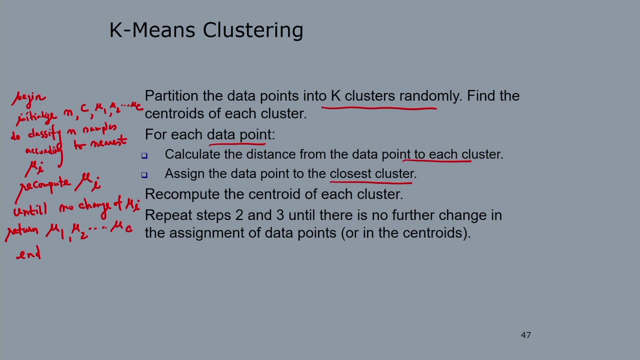 and recompute the centroid of the is cluster that I am considering recomputing until no centroid arrives of the mu, i that I have to do this iteration and finally I will be getting the centroids. the centroids are mu 1, mu 2, mu c, like this. So this kind of concept I can explain in my next slide. 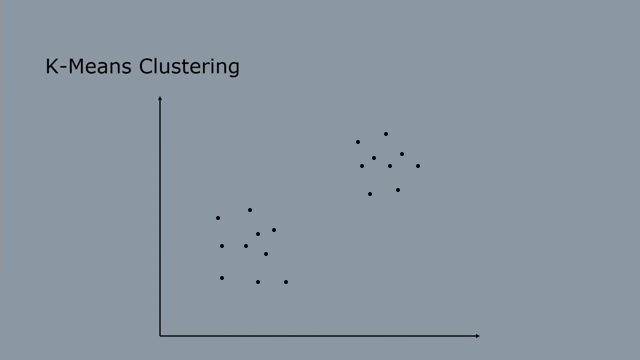 so you can see, I am considering- suppose the clusters are like this- and randomly I am selecting two cluster centroid: one is the red, another one is the green. two cluster centroids I am selecting After this what I am considering. I am considering the distance between the sample. 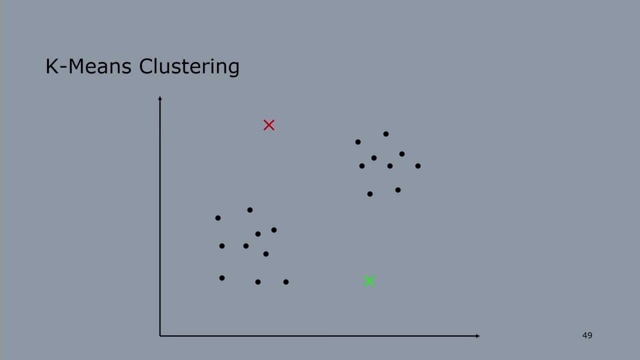 points and the cluster centers. that means the cluster center means the mean. So in this case, by finding the distance between the sample points, you can see this point is assigned to this cluster. similarly, this point is assigned to this cluster. this point is assigned to this cluster like this: 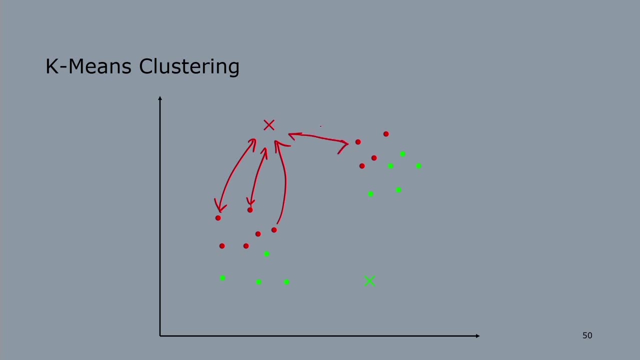 based on the minimum distance, I can determine which sample point is crease closer to a particular mean Similarly corresponding to this point. this point is close to this close to this mean, this point is close to this mean and, like this, I can decide whether this sample points. 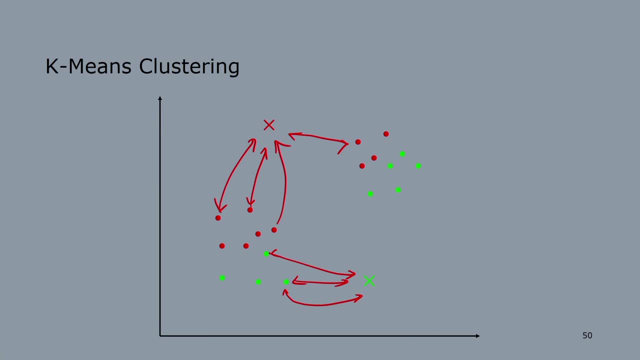 belong to a particular cluster, particular centroid that I can decide. Similarly, this point is closer to this as compared to the red centroid. So, based on this, I can assign the sample points to the centroid, red centroid and the green centroid. After this I have to recompute. recompute the centroid. 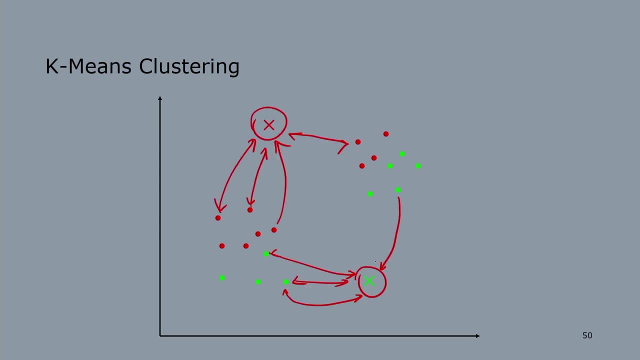 You can see the previous centroid is here and after this I am recomputing the centroid, So next centroid will be this. This procedure I have to repeat again and again. You can see again. I can see whether this sample points belongs to this or this. I have to see. 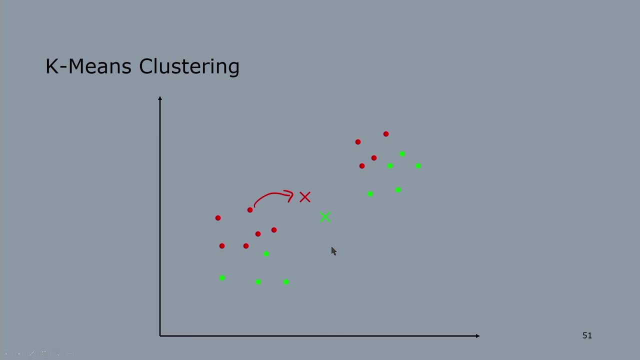 that is based on the distance, I can do this. and again I can see whether this is close to this or this. I have to find like this: And based on this you can see: these two points are now assigned to the red centroid. and again I am recomputing the centroid. I am recomputing the centroid and after this, again like this: 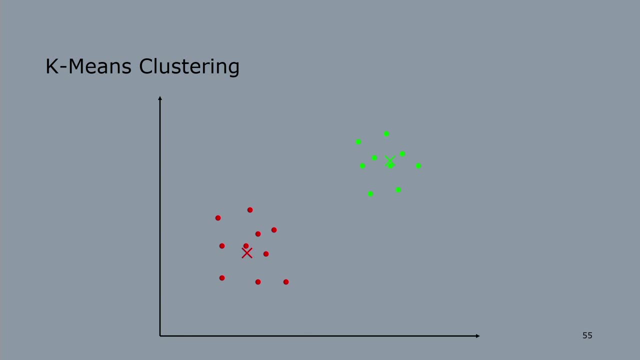 and finally, I am getting the centroid like this and I am getting the two clusters. So this is one cluster corresponding to the centroid centroid is a red centroid and corresponding to the green centroid, I have another cluster. So this is another cluster. This K-means algorithm. 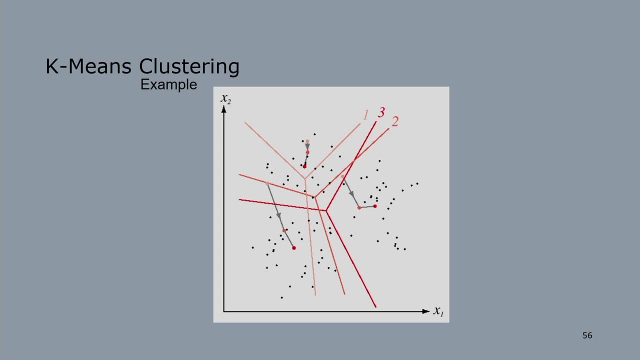 So the procedure I have shown here. So initially I have to randomly define the cluster centroids. that is the mean. After this I have to assign the sample points to a particular centroid based on the minimum distance I can consider the Euclidean distance between the sample points and the centroid. 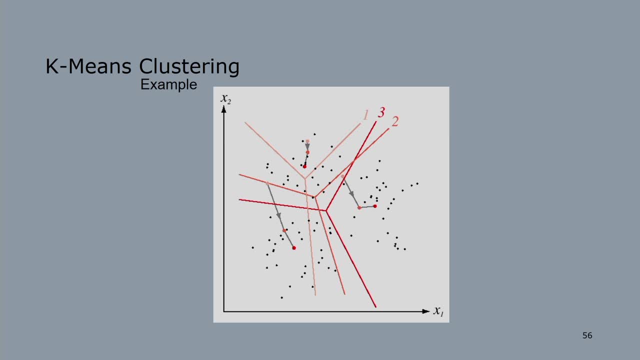 and, based on this, a particular centroid can be assigned to a particular mean, like this I can consider: and finally, if there is no change of the centroid after all this, then I have to stop the iteration and I will be getting the clusters corresponding to all the centroid. 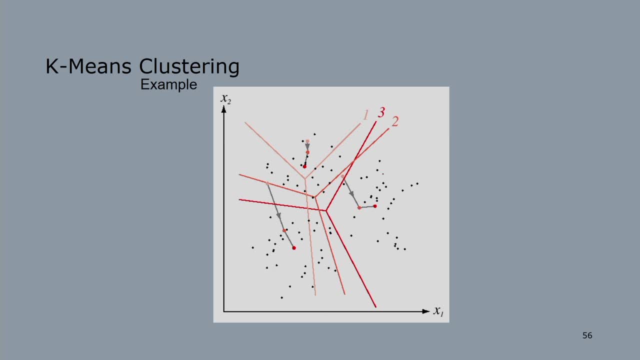 I have to do like this So you can see here in this figure, you can see all the iterations and finally, I will be having the centroid like this. So the centroid will be like this after all the iterations, because I have to update the centroid after each and every iteration. 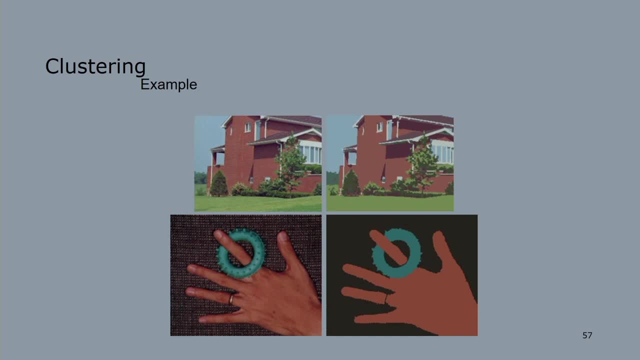 So this is one example of the clustering that you can see. I have the input images. Okay, So you can see I am applying the k-means clustering algorithms for image segmentation. So in this case I have only two clusters: one is this cluster, another one is this cluster. 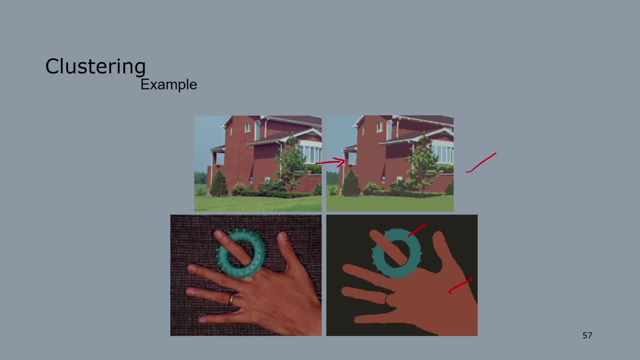 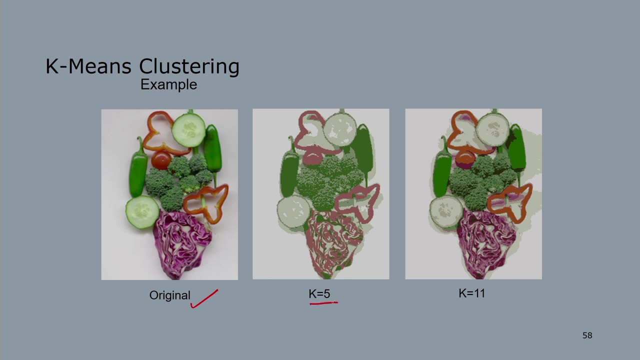 and similarly you can see this is the result of the k-means clustering. I can give another example. this is the original image and in this case I am considering k is equal to 5. that means 5 centroid are considered. and in the second case I am considering k. 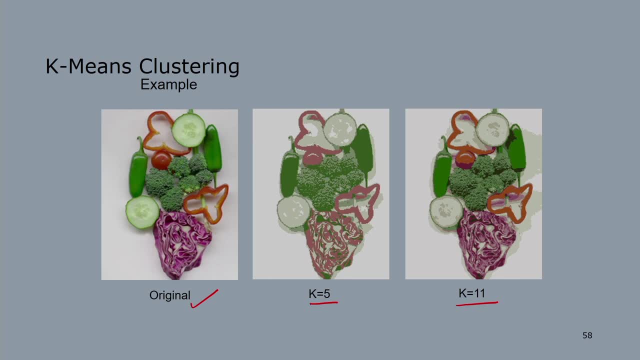 is equal to 11, that means 11 centroid are considered 11 clusters I am considering. k is equal to 5 means the 5 clusters I am considering and corresponding segmented images. you can see in the results. This is about the k-means clustering and also I can use the motion for image segmentation. 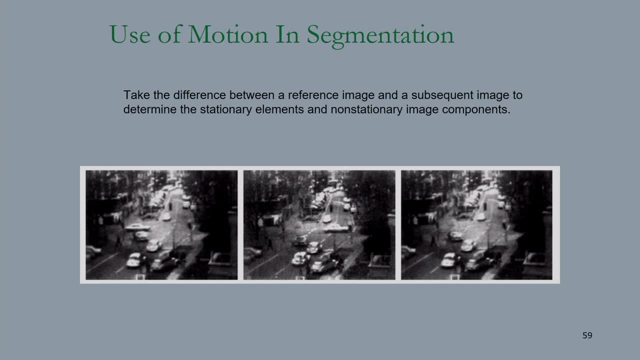 So just I am giving one simple example. suppose I am considering one video sequence and suppose this is one frame and this is another frame of the sequence and you can see one moving car is there. You can see one moving car is there. and if I take the difference between a reference, 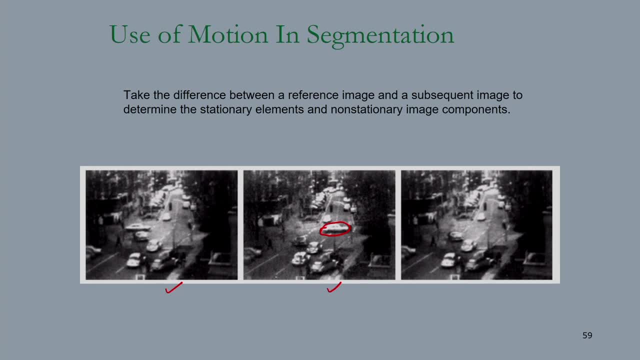 image and the subsequent image, then what I will be getting. I can get the stationary elements and also I can determine the non stationary elements. So in this case, one moving car is here available and in this case this corresponds to the stationary elements, the stationary background I will be getting. 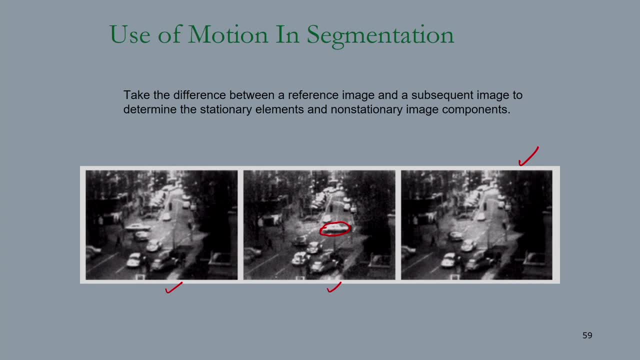 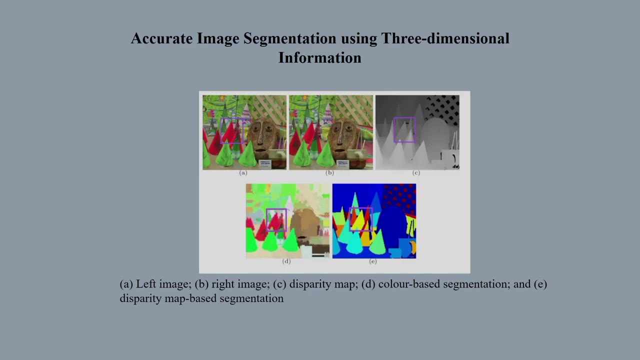 So this is the concept of the motion in segmentation. Just, I am taking the difference between the reference image and the subsequent image Of the video sequence to determine the stationary elements and the non stationary image components that I can determine, And also in stereo imaging, you know, I have the left image and the right image and we 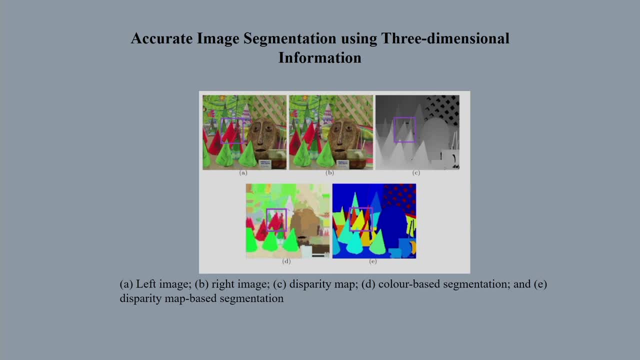 can determine the disparity map and from the disparity map I can do the image segmentation. So here you can see: the first one is the left image and the right image is the non stationary image. The second image is available and I am calculating the disparity map here. 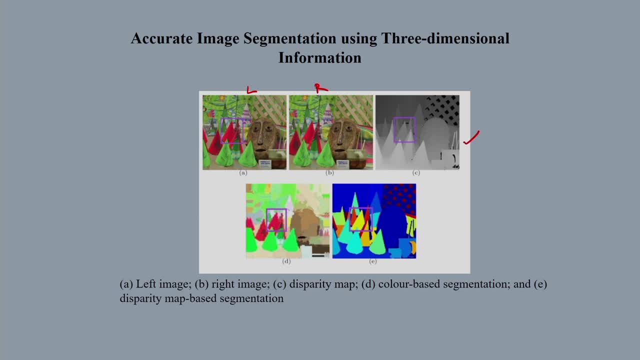 C is the disparity map and based on the color I can do the segmentation. So D is the result of color based segmentation and E is the result that is obtained from disparity map based image segmentation. So I can also use disparity information for image segmentation. 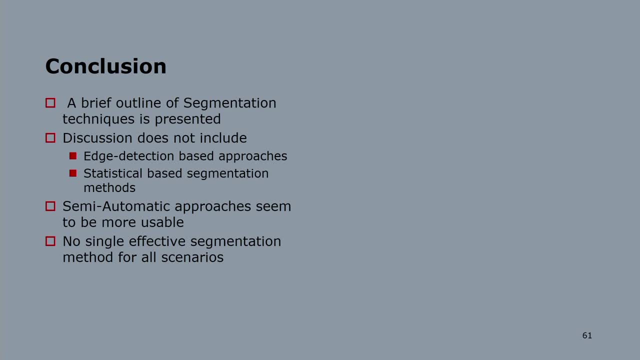 So briefly I have outlined the segmentation techniques, The edge detection techniques, The image segmentation techniques. Segmentation based approaches, The statistical based segmentation method, are not considered here in this discussion, And one point is that no single effective segmentation methods for all the applications.